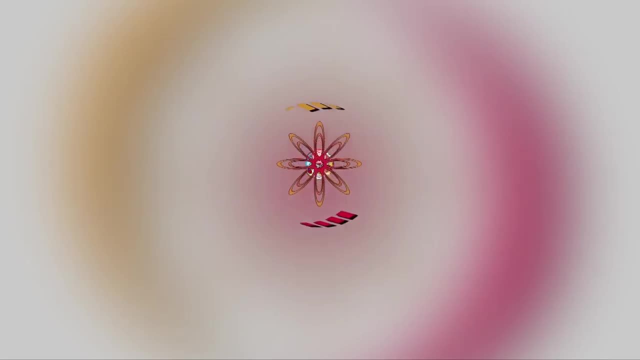 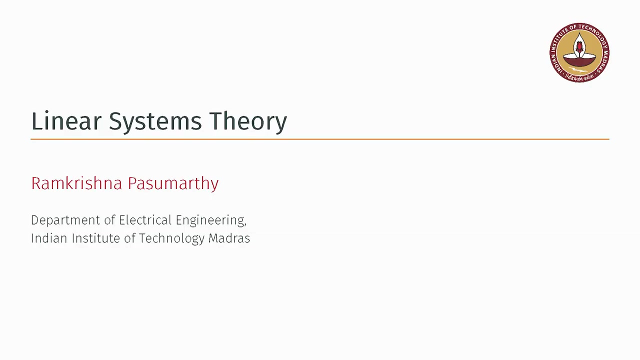 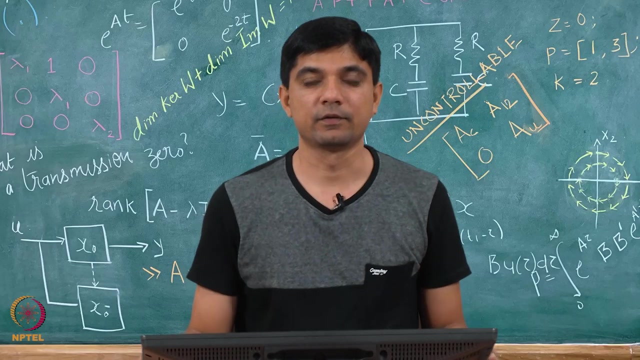 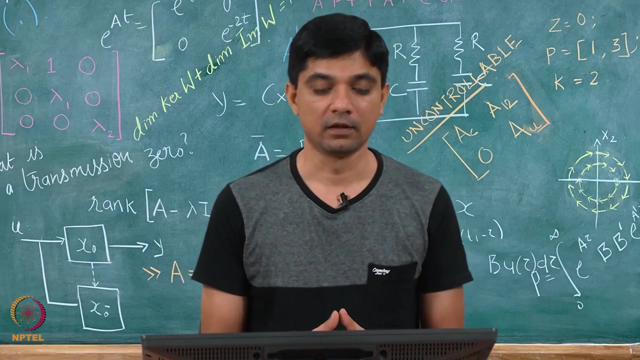 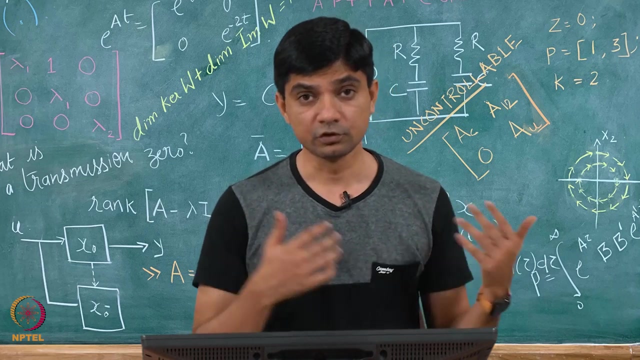 Hi everyone. So welcome to this week 11's lectures on the course on linear systems theory. I am Ram Krishna from IIT Madras. If you have survived this course till week 11, I think you are doing pretty good. So just a very quick recap of what happened over the past. 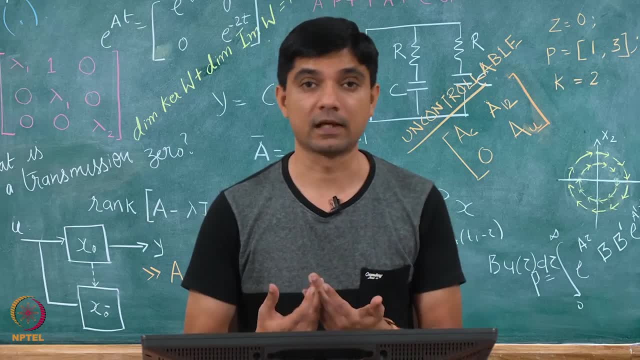 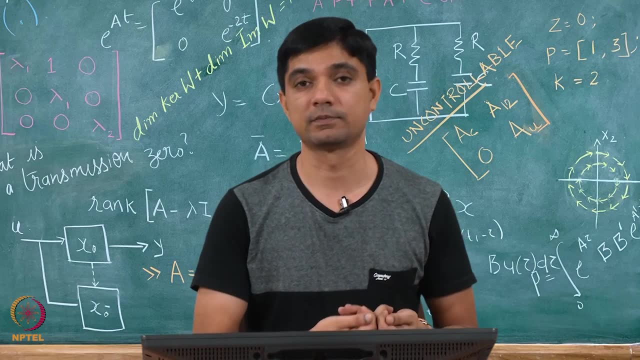 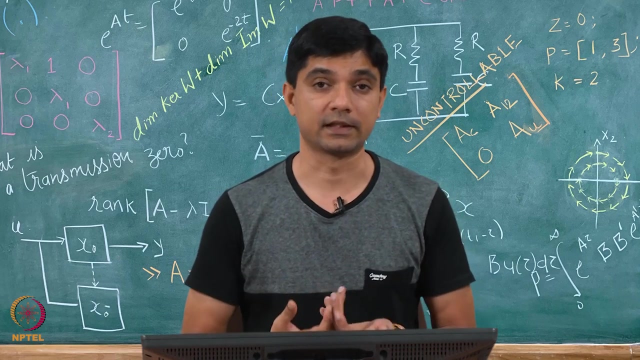 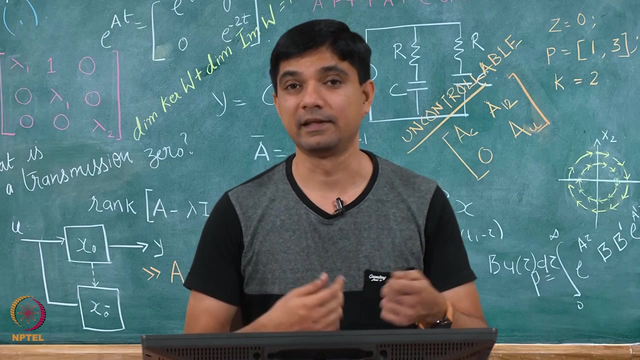 two or three weeks was at least from the design perspective. we had formulated design problems, as certain say, pole placement problems, or we also at some point of time asked ourselves a question: what if the states are not completely measurable? then we had an equivalent observer design. We also looked at simultaneous controller and observer design, and so how a design of 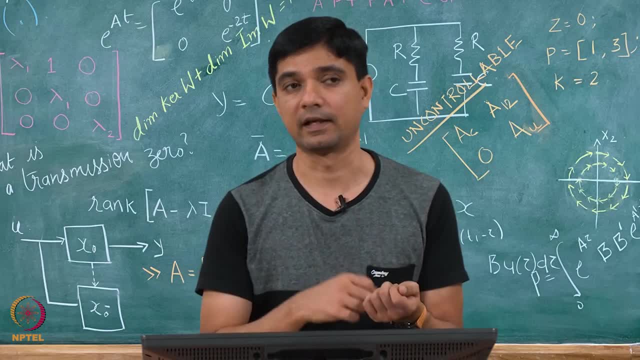 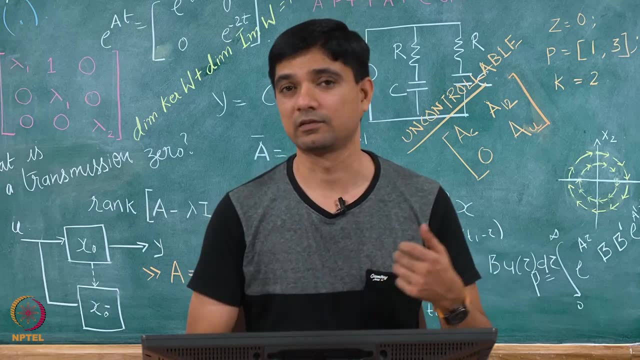 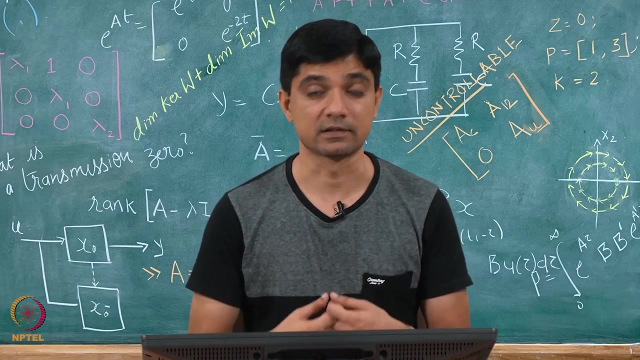 a controller does not really affect what is going on in the observer design and vice versa, So this can be treated as independent problems. and how? also? towards the end, we saw that the observer dynamics should be faster than the controller dynamics for obvious performance reasons. ok, So what we were interested in? We were interested. 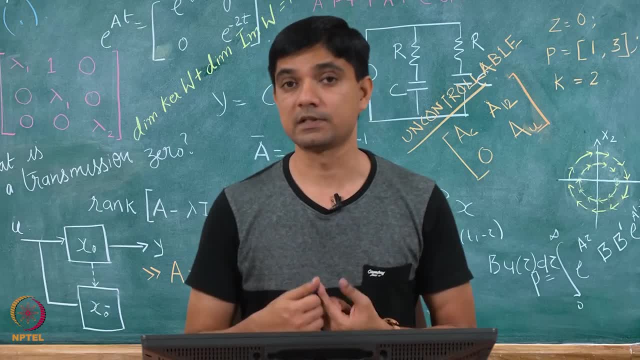 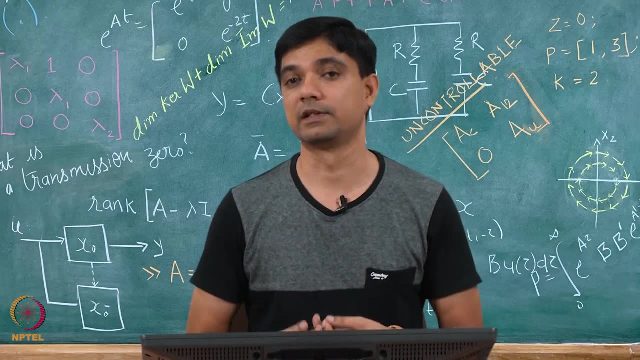 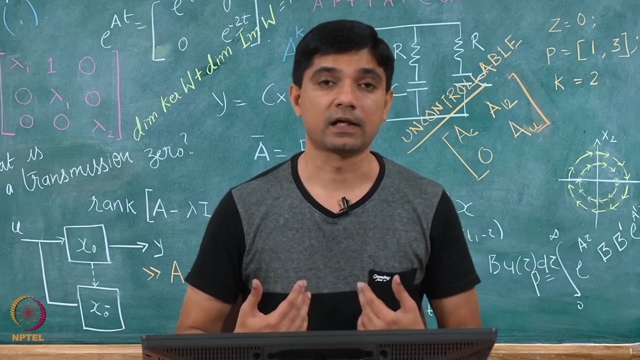 in one stability. Second performance in terms of placing the closed loop poles at desired locations and, of course, at times when we required an observer design, we actually also followed the procedure of designing the observer And starting from the definition of controllability right. So 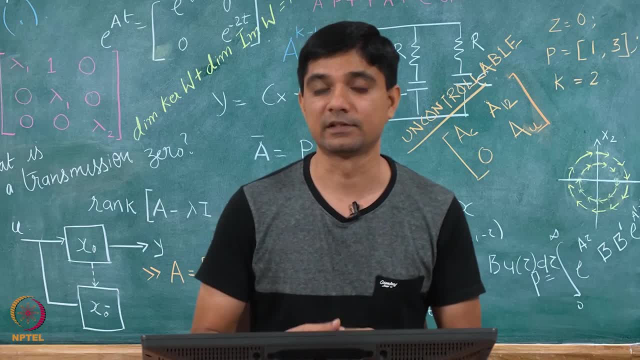 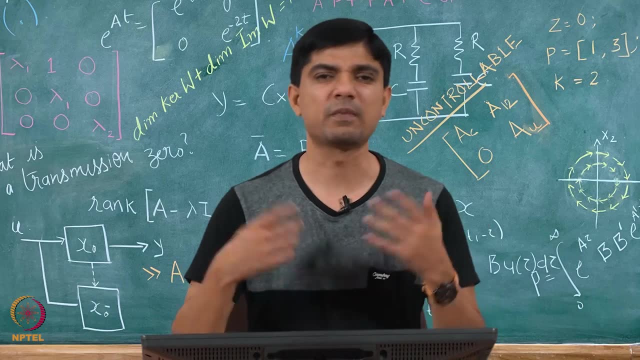 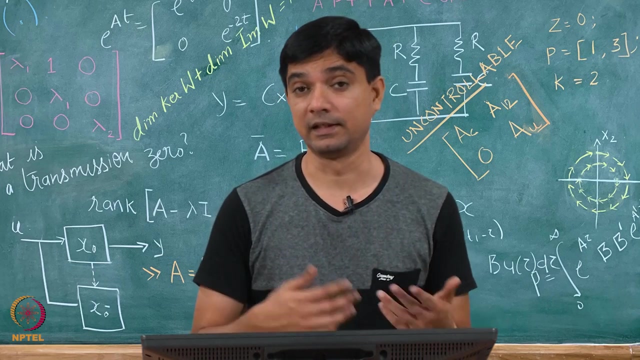 loosely speaking, we. so the control definition was: can I start from any point in the state space and come back to the origin with help of some unconcern? I was not really interested in what is the control effort required or how much time does it really take. I was just happy saying: well, it should reach from point A to point B in. 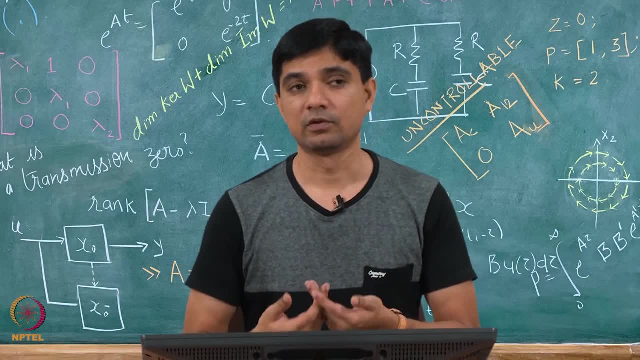 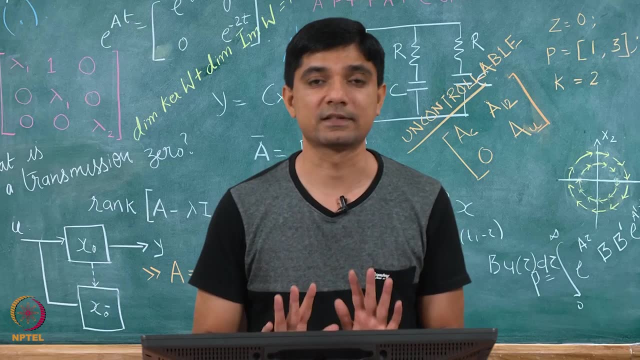 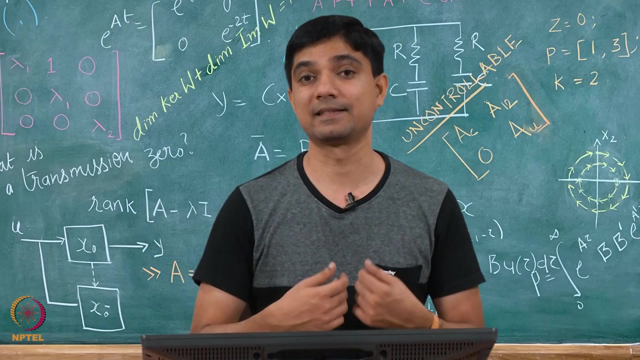 some finite time right and also an unconstrained control input. So we are only interested whether or not the system is, say, for example, controllable. We never talked about what is the cost of the control in what? so, can I say, with a control? 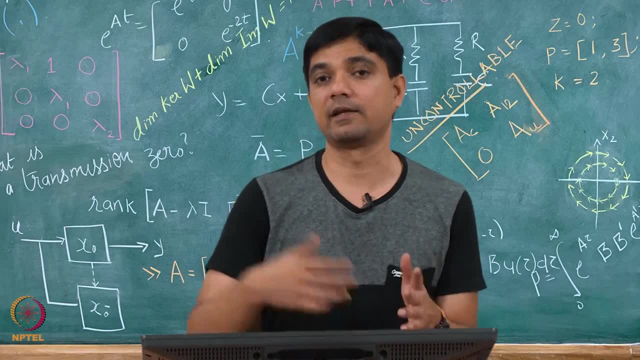 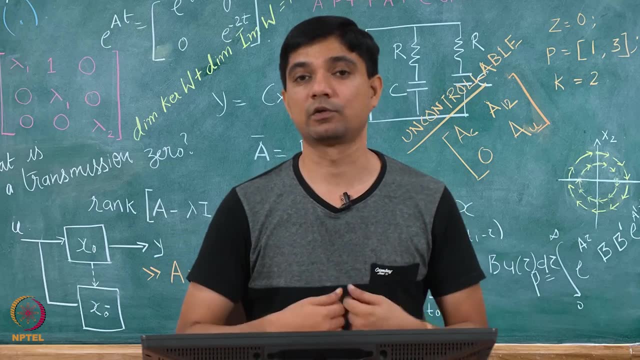 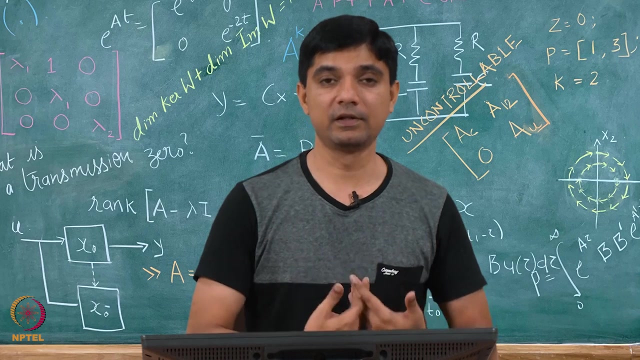 restricted to some quantity. u bar, can I reach from point A to point B in, say, some 5 seconds, for example? right, We never really talked about quantifying those quantities, right of the inputs, the time and so on. So what we will today do is to look slightly beyond just pole placement. 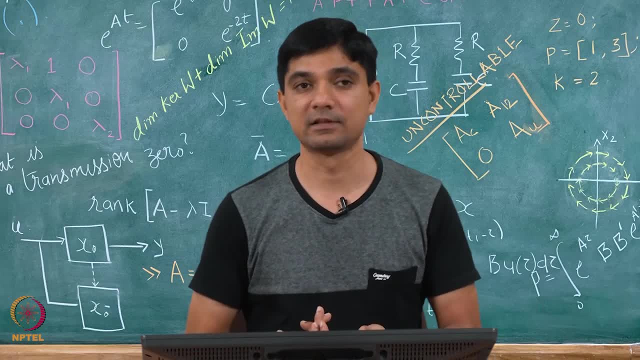 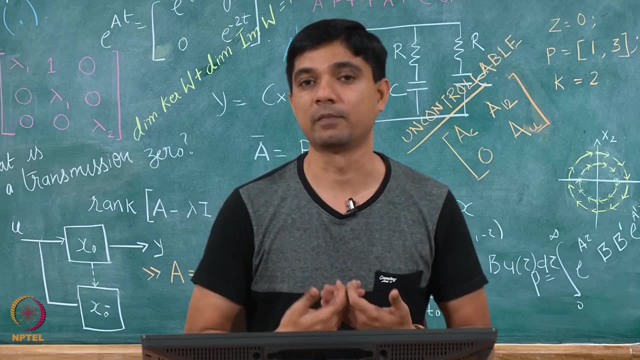 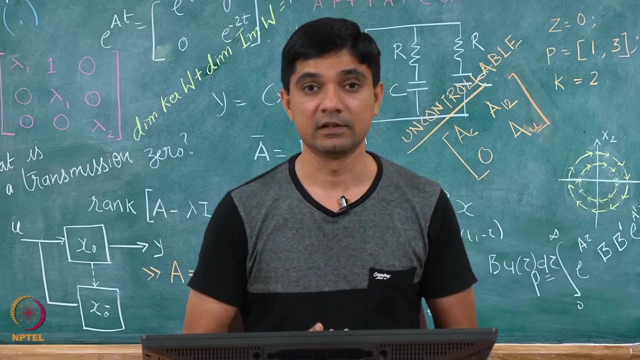 So pole placement, or just beyond, looking at stabilization kind of properties, or beyond looking at just a control problem, as just u equal to minus kx, such that the poles of the closed loop system are at the appropriate locations. So we will do something slightly different today and of what is called as an optimal. 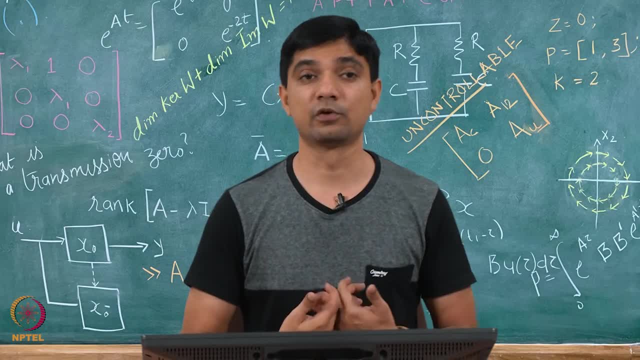 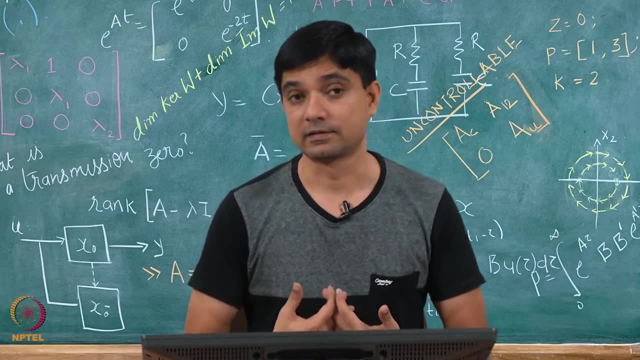 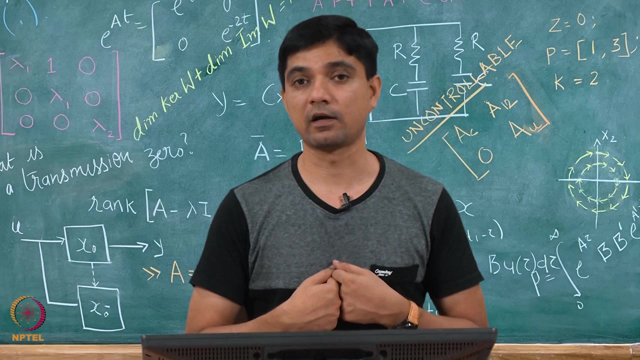 control. So what is a good control law? A good control law is something, Is it is an expensive control law. good control law right is? it is like if I were to draw an analogy to check what is a good car for me to buy. ok. 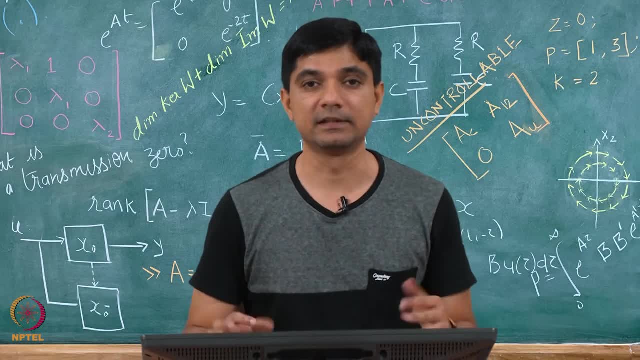 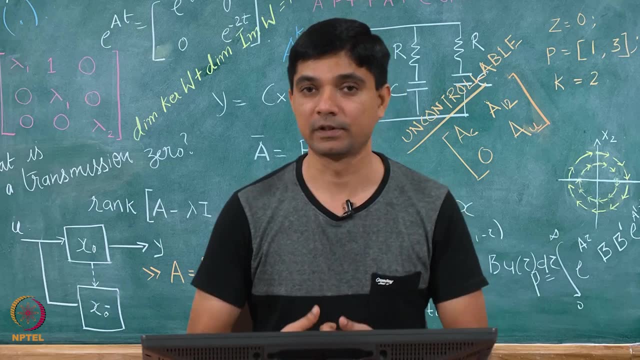 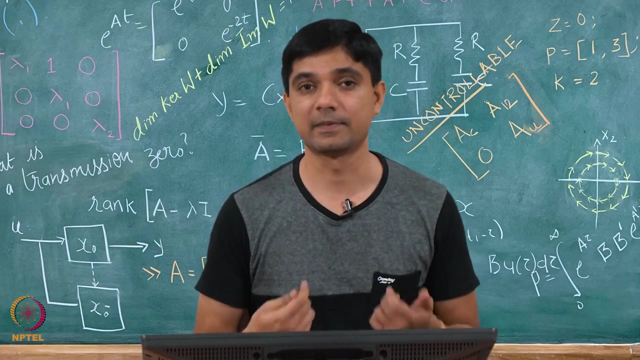 Then you just, maybe just out of curiosity, just ask Google or you ask Alexa, for example. she is also quite competent these days of what is a good car and that in sometimes is also not. So it is not a well posed problem, because you do not really specify your requirements. 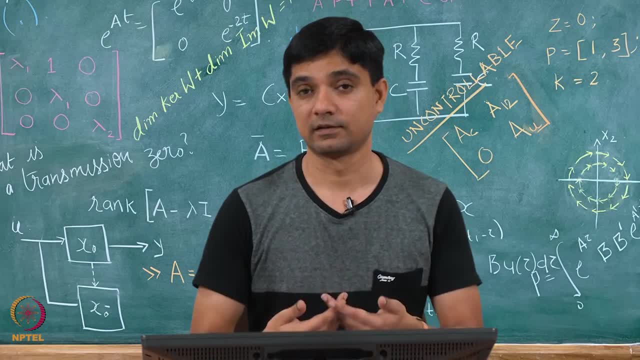 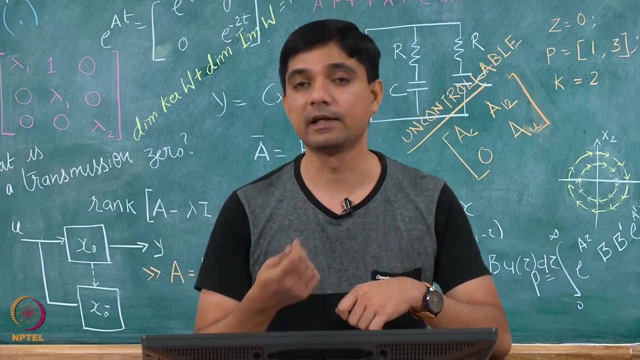 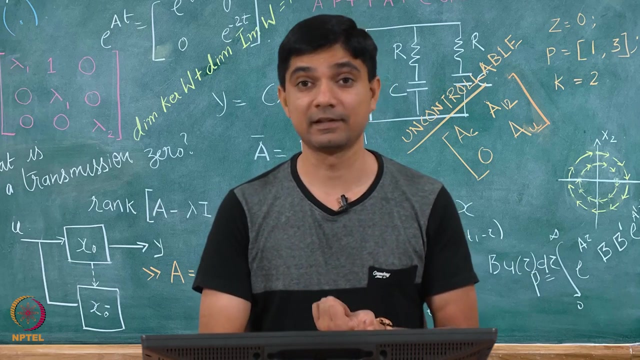 of: why do you need a car, what is, what is the cost that you can afford, and so on. It is also looking in a different way if I say: I get a salary per month. I want to maximize my savings. I also want to maximize my comforts, right? 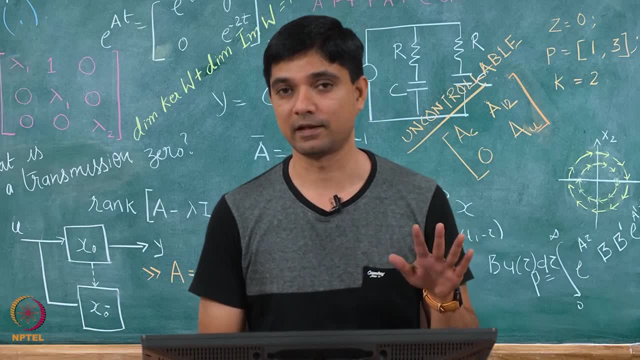 So what is a good solution? So if I say, well, I want to maximize my savings, I also want to maximize my comforts, right? So if I say, well, I want to maximize my savings and I should not spend at all, or if I say I 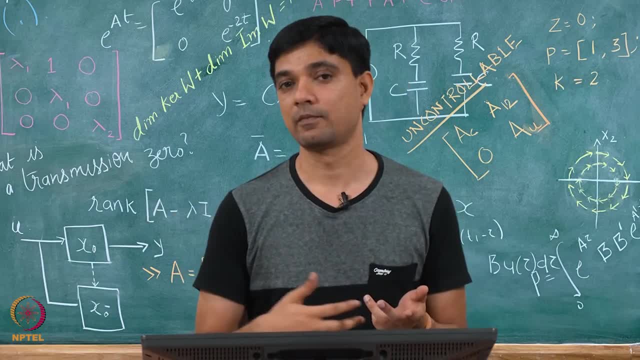 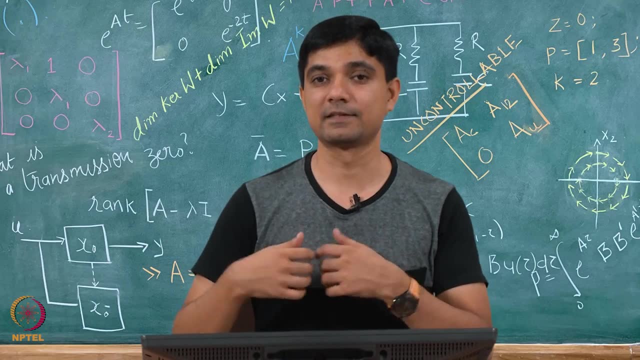 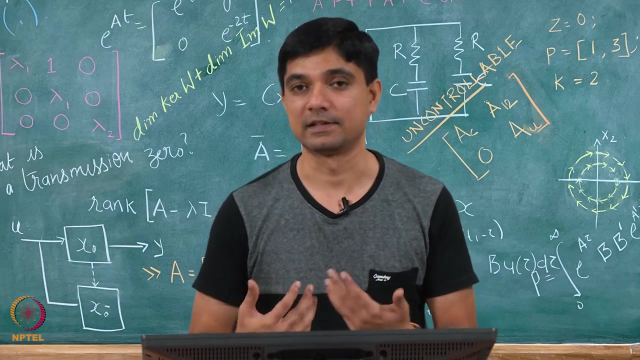 want to maximize my comfort or luxury levels, I should not save at all. So this is like in some sense a contradictory problem: right of maximizing my savings versus maximizing my comfort levels. So what does that mean in the control sense right? can we actually solve problems like 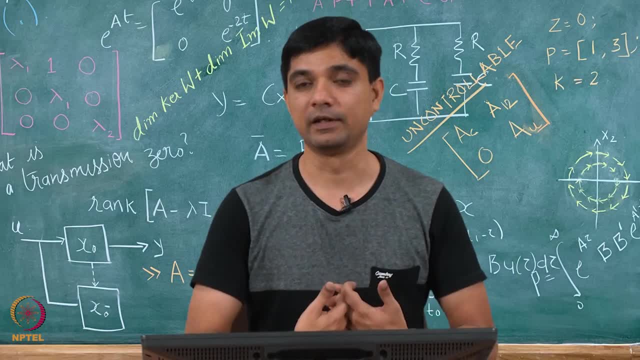 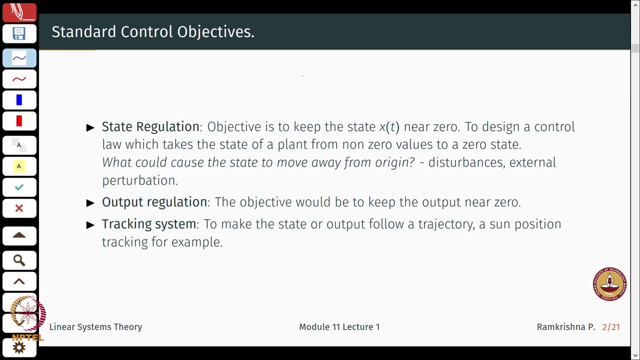 this when we have a conflict between good performance plus some constraints which occur to us. ok, So what are the control problems that we typically encounter? or say So? one is what we call as the state regulation problem, which is to keep the state x near 0, right so to. 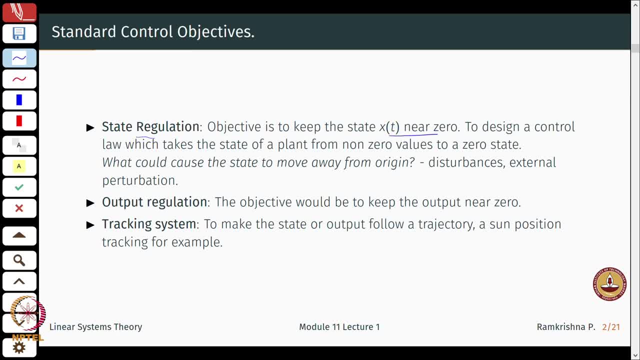 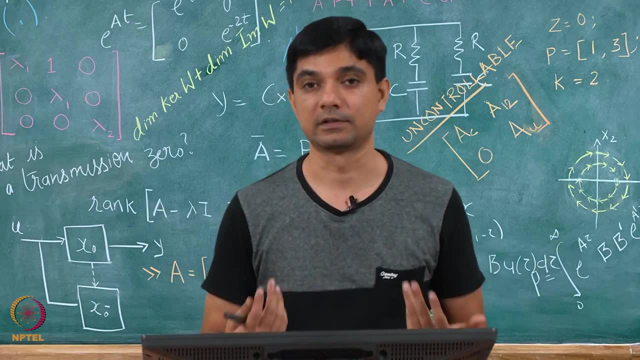 speak. So what is the aim of the controller? Aim of the controller is to design a control law which takes the state of a plant from some non-zero values to the zero state equilibrium, for example. Now well, why does this actually occur? Why do I even need to design the controller? 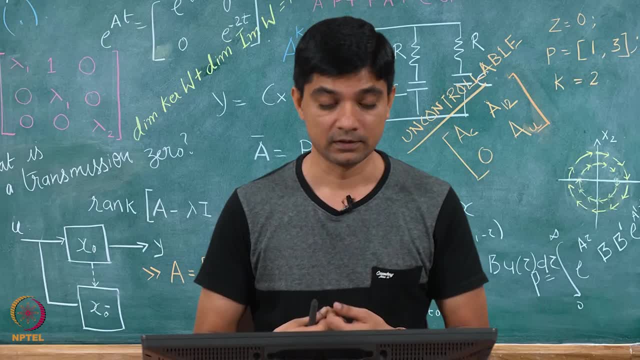 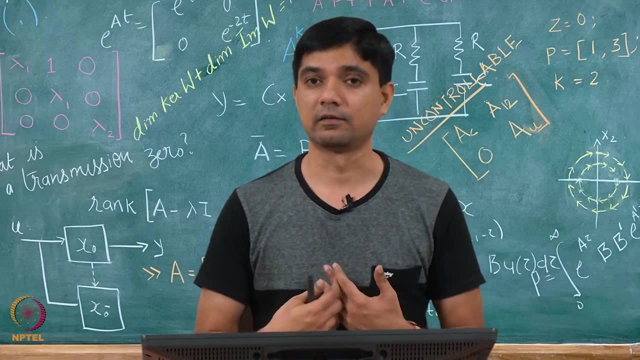 So if I am at the equilibrium, I will always be at the equilibrium. So what would cause the state to move away from the origin? There could be disturbances. there could be external perturbations. say, if I am looking at a power grid, a sudden change in load patterns might. 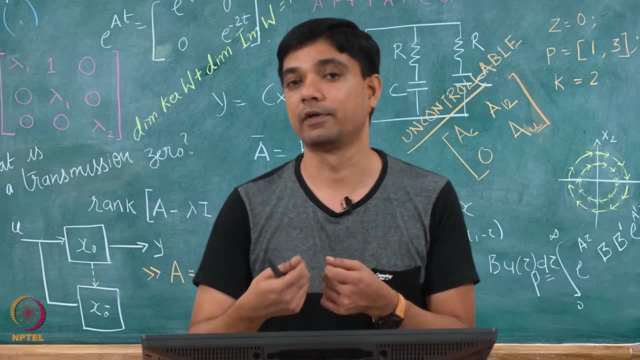 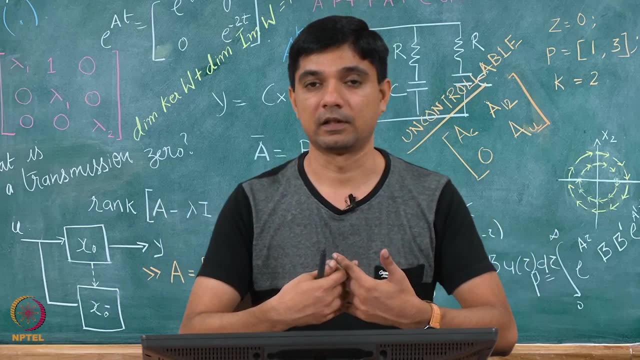 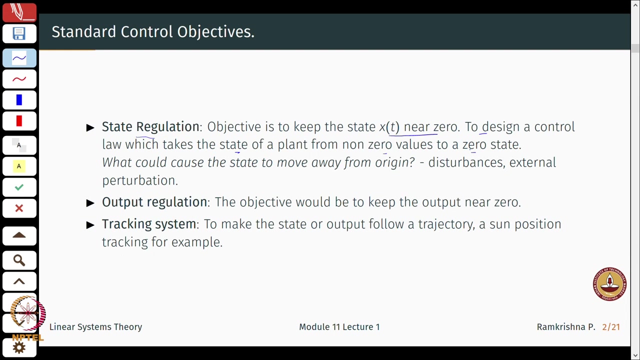 actually Trigger my system in such a way that it will move away from the set point. or if I am looking at IRCTC website, a sudden a booking pattern might take my system away from my set point, so to speak. So we can also- we can also similarly look at not only state regulation but output. 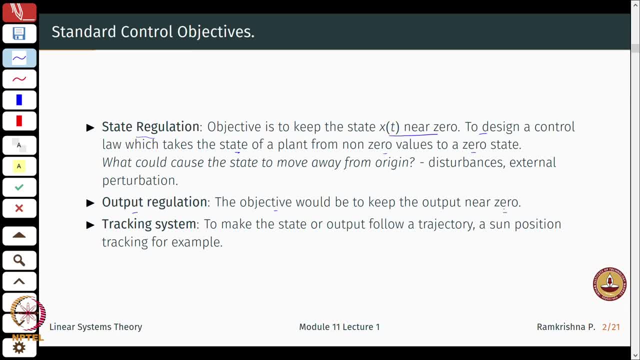 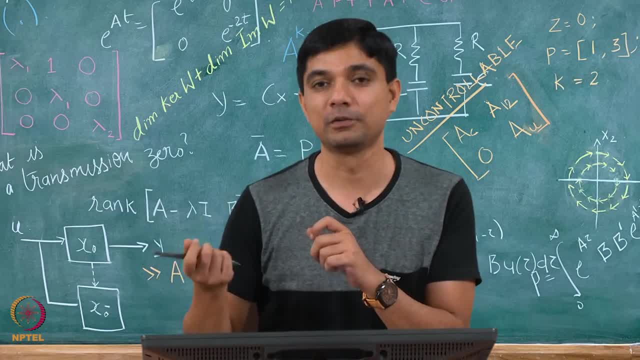 regulation where the objective would be to keep the output near 0 or some. So the 0 is that I do not want to really drive the system to a 0 output, But some kind of a reference value which I set and you know where usually you can also. 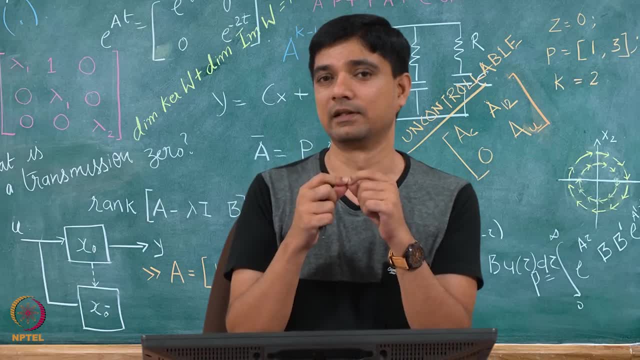 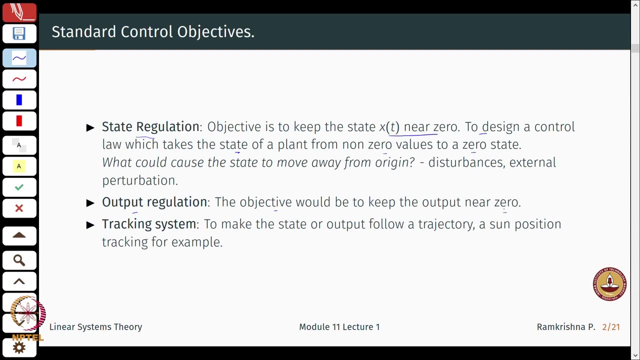 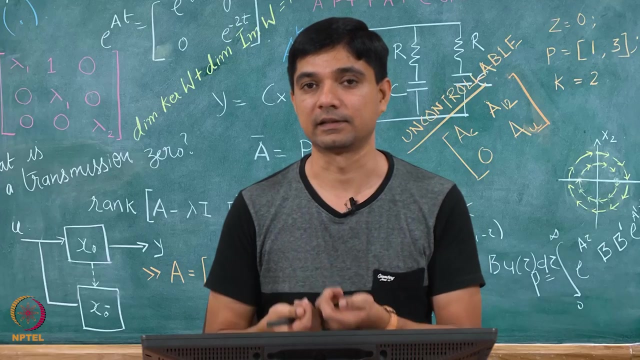 talk of it in terms of the error being, you know, in towards, towards 0,. ok, Now the third thing could be looking at a tracking problem, right, where I can make the state follow, or even the output, in some case follow a desired trajectory, say I am, I want. 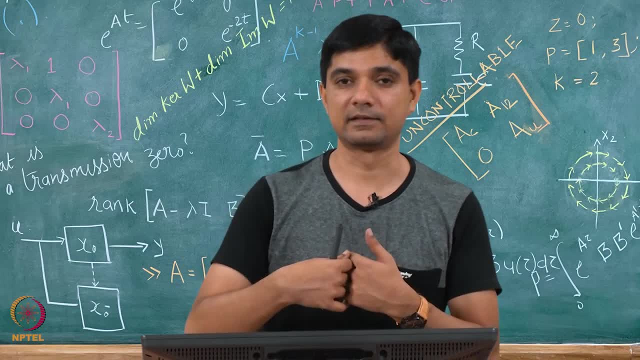 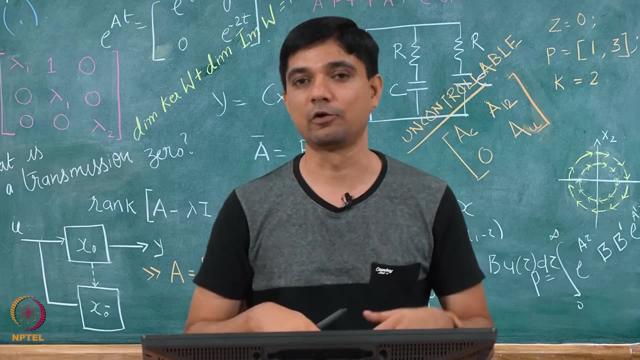 to design a solar panel then it seems. So if I would maybe phase it at the input point east in the morning towards the end of the day, I may not maximize the output of my, of my solar generator, right. So I have to really track the position of the sun and this has. 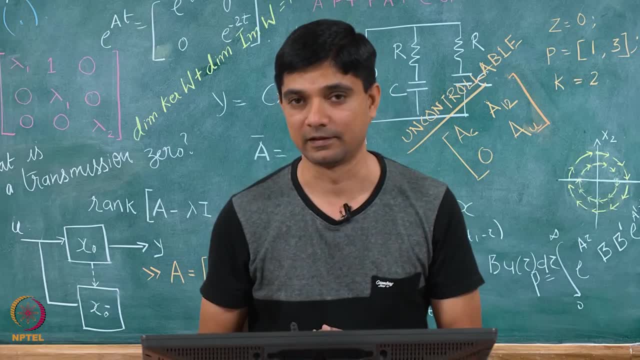 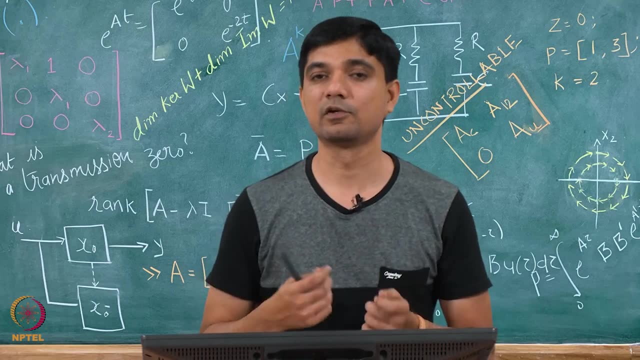 been kind of a very interesting and well studied problem in control literature or even from power engineering perspective, right. So these are typical control problems that we encounter. So so far we are like: can I design a controller u equal to minus kx such 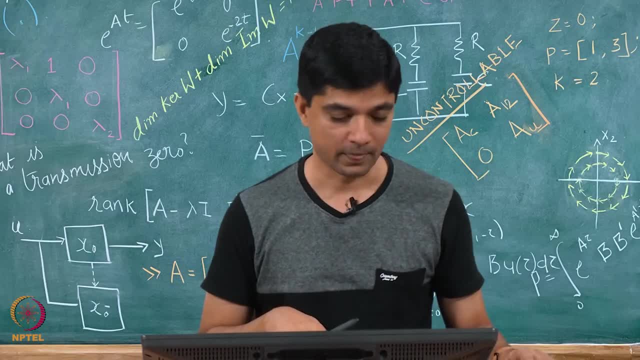 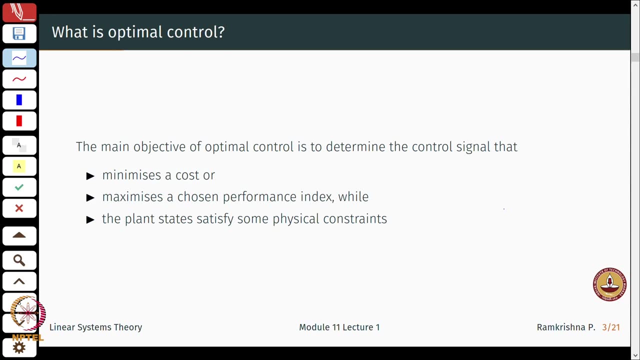 as that poles are blah blah blah, performances blah blah blah and so on. ok, So when I look at a little further, yes, I can design a controller, but now I need to answer a little more questions, right? So one question would be well, the main objective? 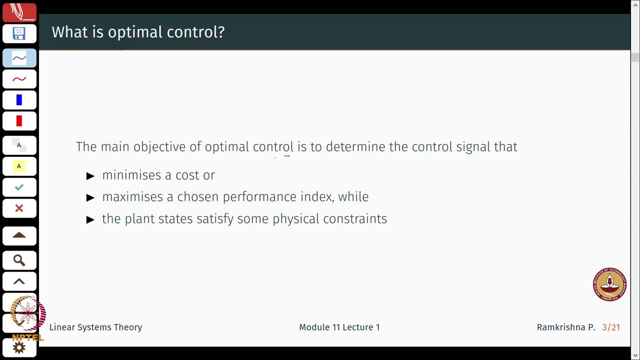 here. if I look at an optimal control, is to design the control signal that minimizes a certain cost right. At the same time, does it maximize a certain performance? Does it minimize a certain point? Does it maximize a certain point? Does it performance index? and the plant could have some physical constraints, Let us say for 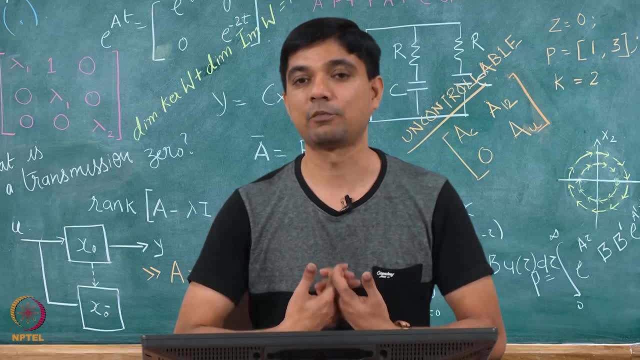 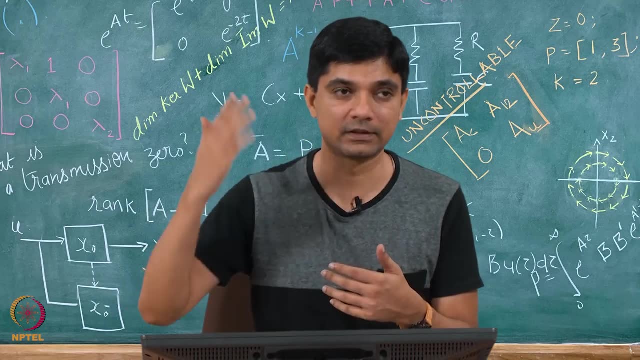 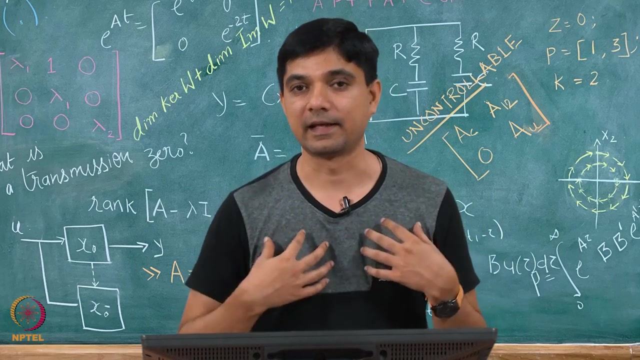 example, if I drive a car, I know that I possibly cannot go beyond, say, 150 kilometers per hour or 200 kilometers per hour. It just comes with some kind of a physical constraint. So even though the car can move, as a controllability analysis would suggest that the car can go. 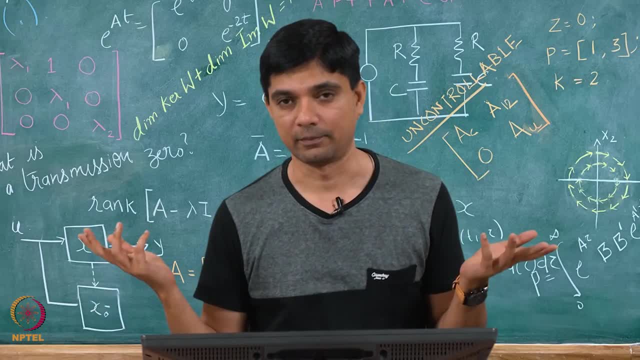 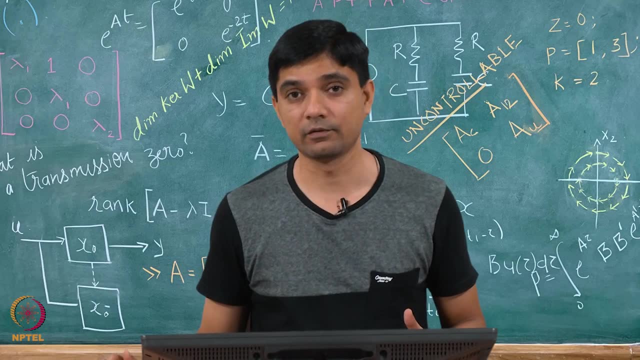 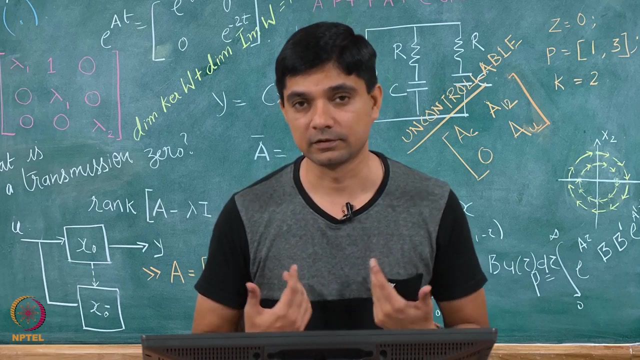 from point A to point B in some finite time. ok, Now if I say, can I go from, say, Chennai to Delhi by my car in, say, 2 hours? well, that is a difficult question to answer, right, As the answer may always not be possible because my car is physically constrained by its maximum. 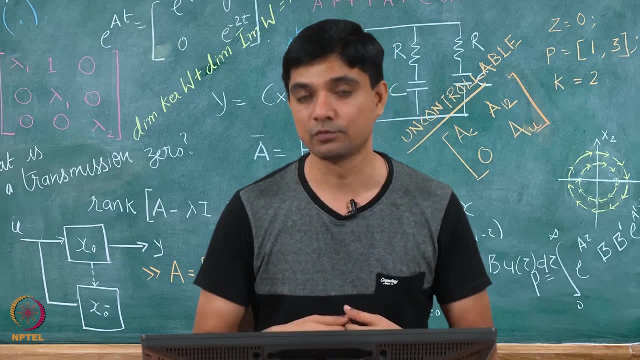 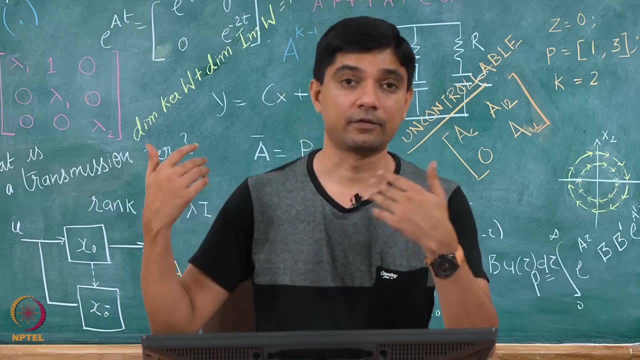 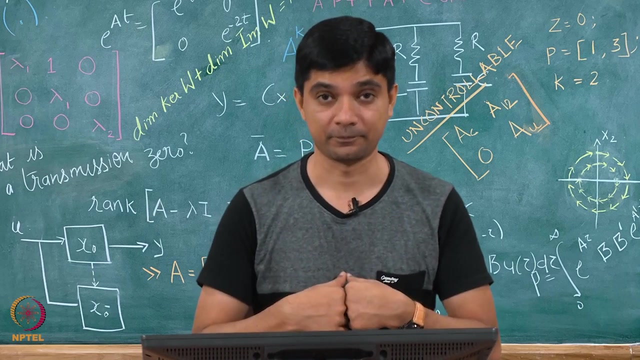 speed, Then in most cases I also want to maximize a performance index. Performance index could be in terms of, you know, say, if I go back to the web server problem which I, which we had in the week once lectures, can I serve maximum requests per second right And not only that, can I also serve request. 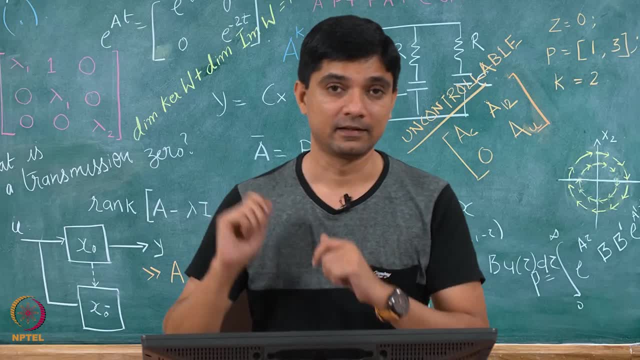 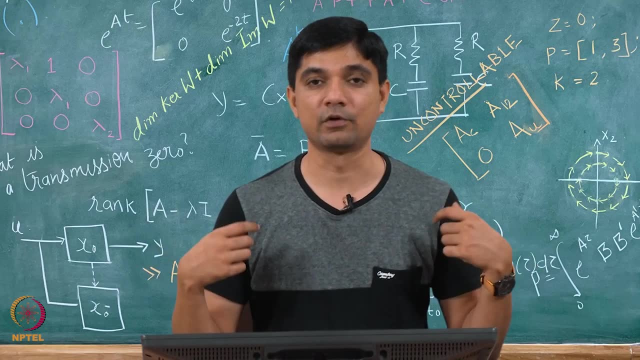 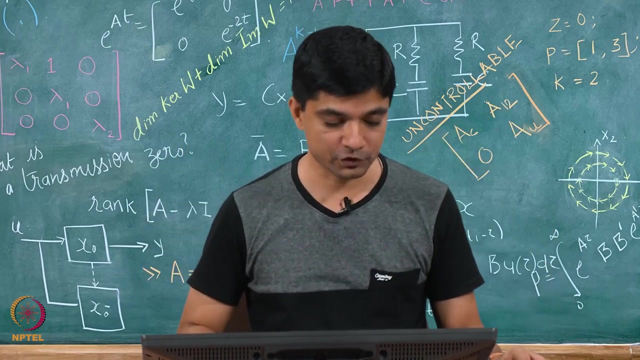 as fast as possible. There was a contradiction also in that particular problem, right? And then of course I want to minimize the overall cost, right? So ideally I would want a maximum performance at 0 cost, right? that is like the ideal situation, Well, but unfortunately that. 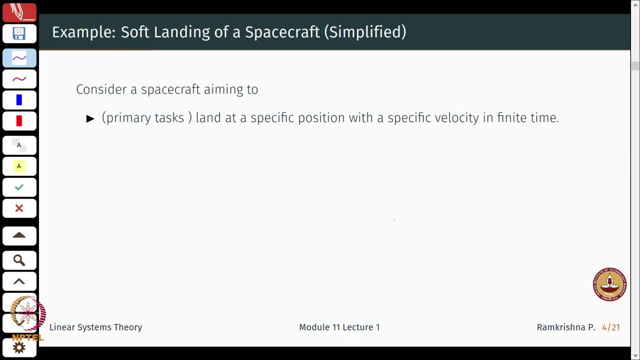 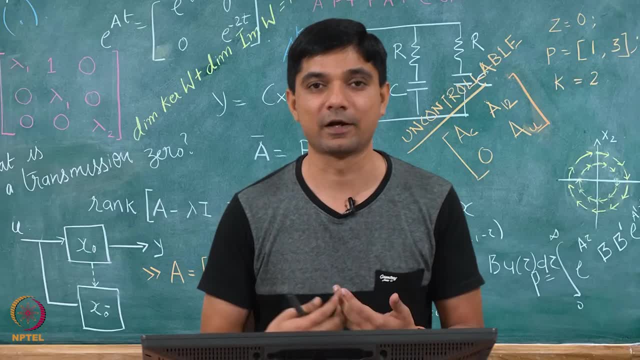 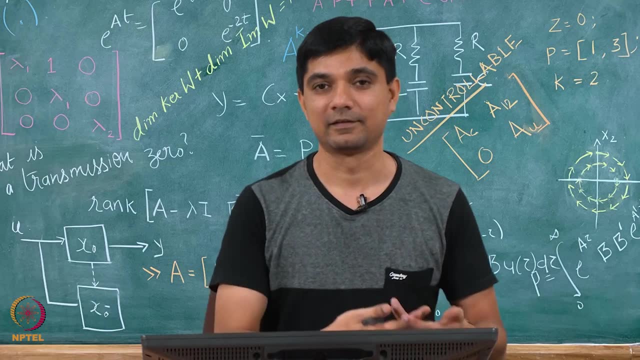 does not happen. So is there something that will help us a bit in this? ok, What could be other examples? So, something which is being talked about everywhere is about soft landing, so to speak. ok, So I will not tell you why we could not get to a soft landing. 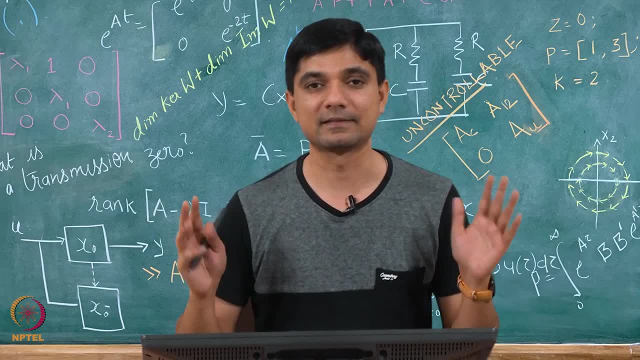 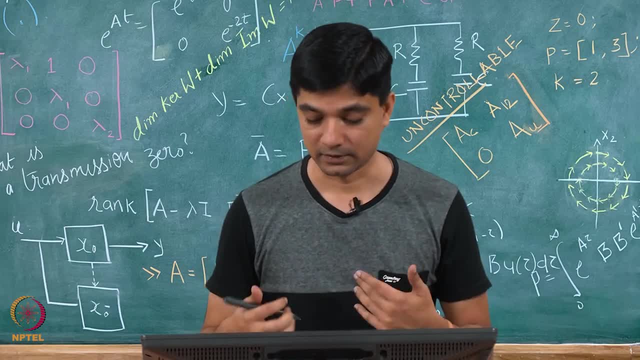 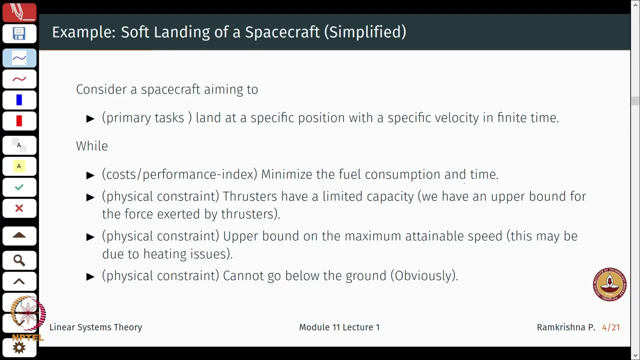 to be the case. So if I just draw some parallel between what actually seems to be the case, that rating, right. So these are essentially physical constraints which come with the system. ok, Now of course, there are another physical constraint: you cannot go below the ground, right? this is kind of obvious. but this is 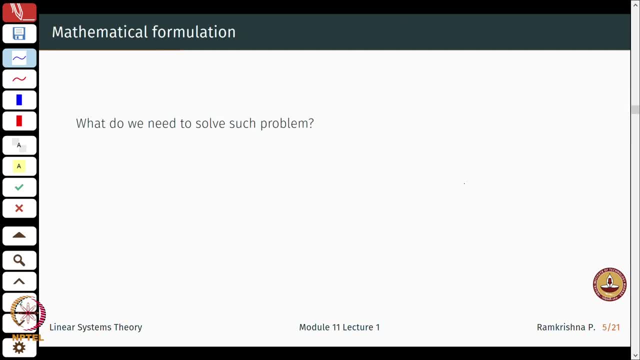 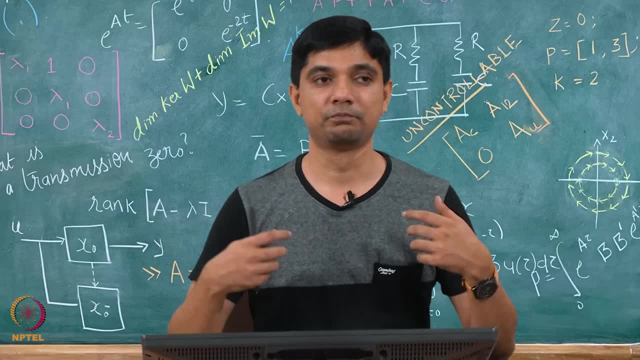 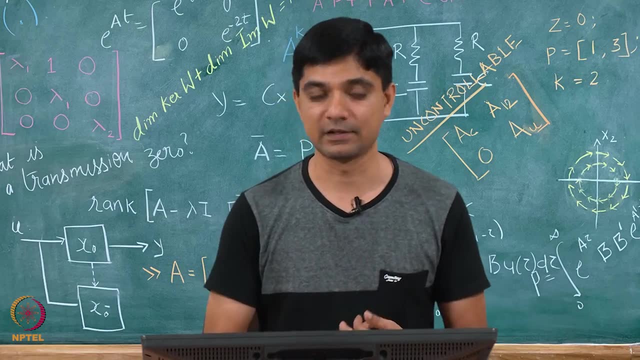 an real time physical constraint. ok, Now, what do we need to solve such problems? It is kind of fancy to talk about this problems of what they call also as soft landing and so on. What do we need to solve such problems? Well, we, from our control engineers perspective- 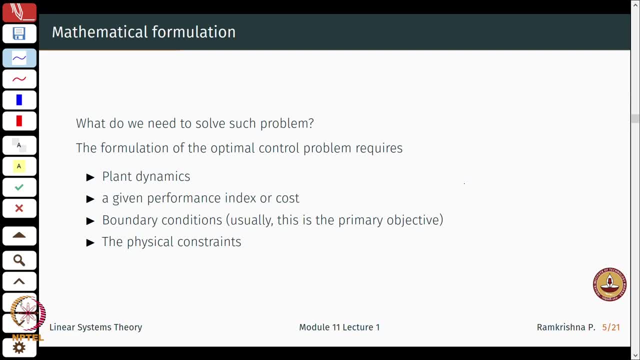 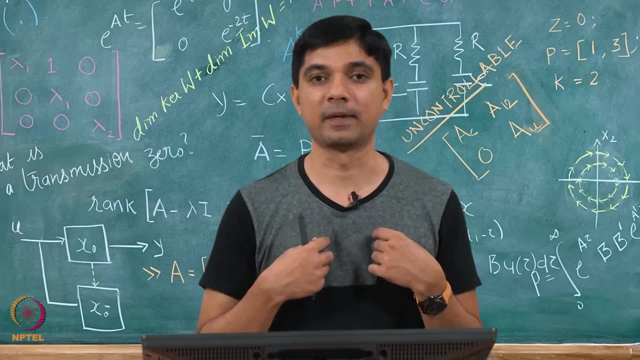 we need a few things. right, I need some few information. First is I should know the plant dynamics as closely as possible. I need to know what is my performance specification. ok, For example, my performance specification as a teacher should be on my teaching abilities. 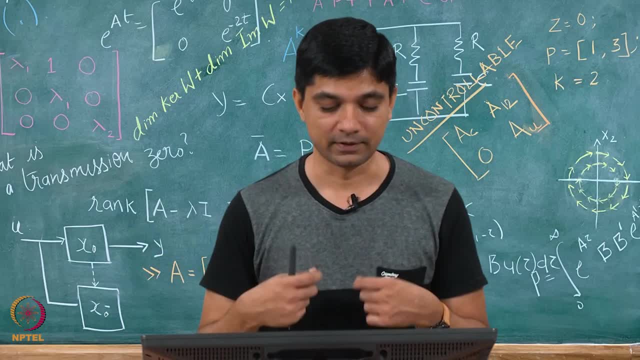 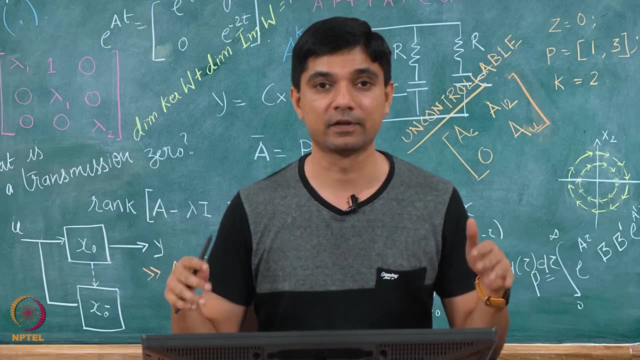 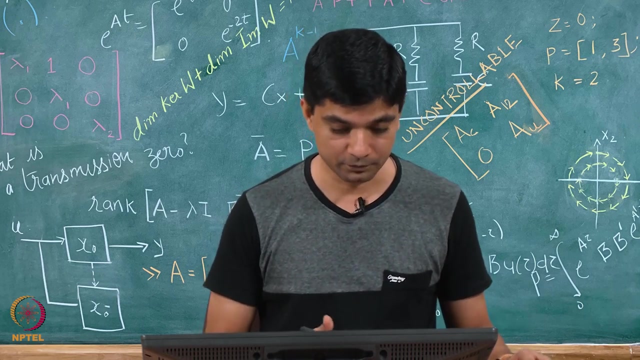 but not my football skills or lack of that, right. So, given a performance specifications, boundary conditions, right. what are my limitations of what can be worked out, what cannot be worked out? right, and then, of course, physical constraints of the system, right. So, in general, 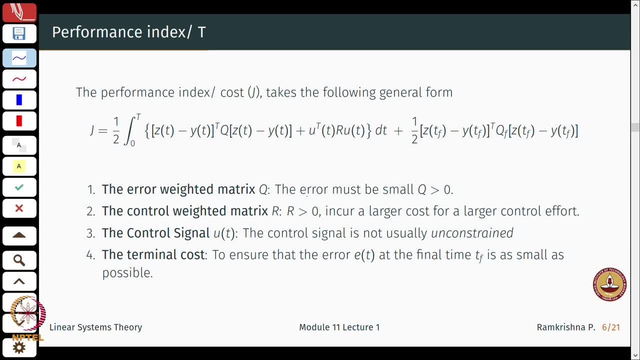 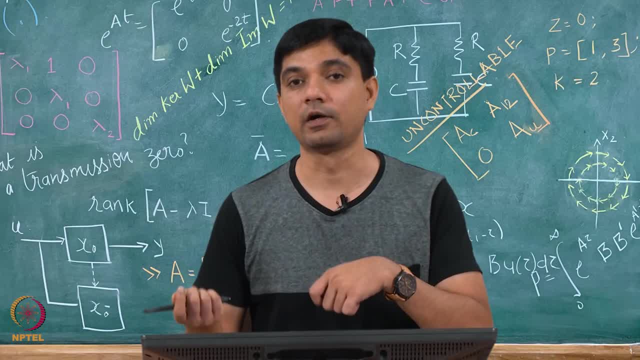 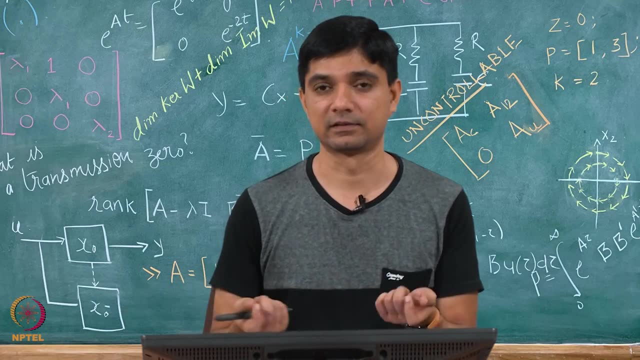 if I were to look at formulating this problem mathematically. So all the time, what we were interested is: given a physical system, can we write a model of that? a model was a mathematical abstraction of the system in terms of linear ordinary differential equations. in this, mostly in this, in this course right. 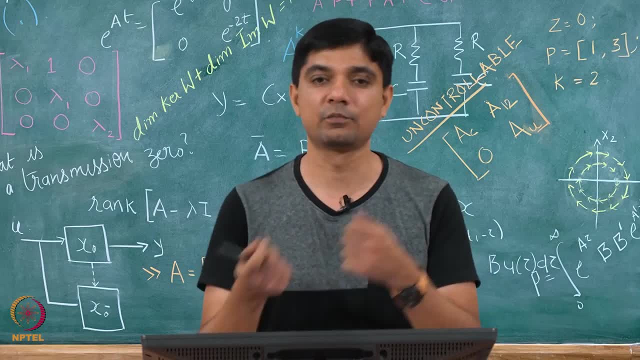 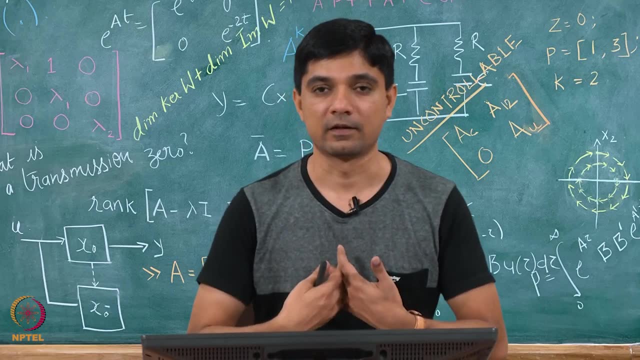 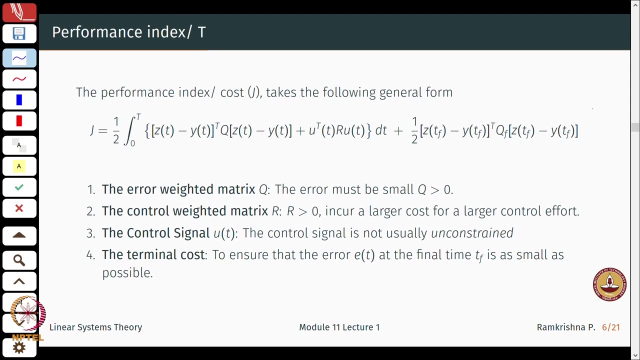 So from that model can I derive a controller and then put it back to my original physical system? that was my very straight forward. you know design procedure in a set, in a simplified way. ok, So let us say one of the more general forms of cost function. I think different, different. 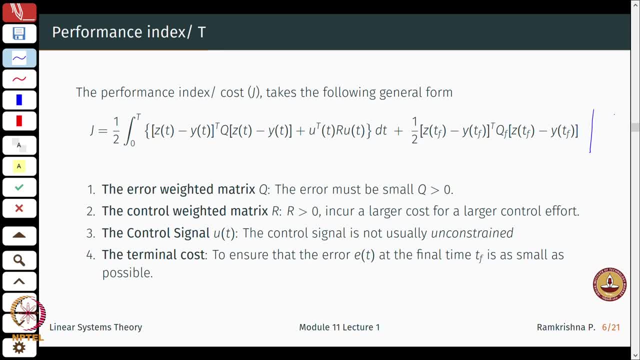 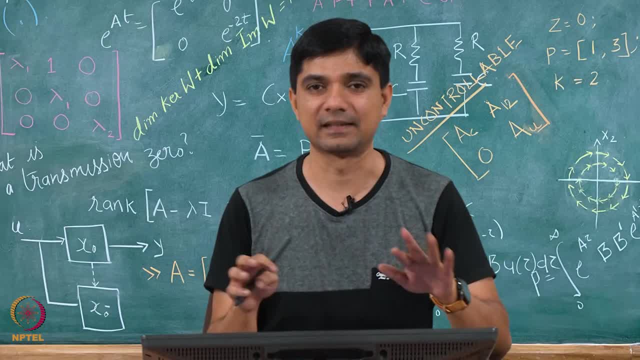 books will will start with different motivation, because we are not really doing an optimal control course here. but this is just a little introduction to optimal control. you are just like- not even like scratching the surface, you are just maybe watching this, the surface, a bit from from this. 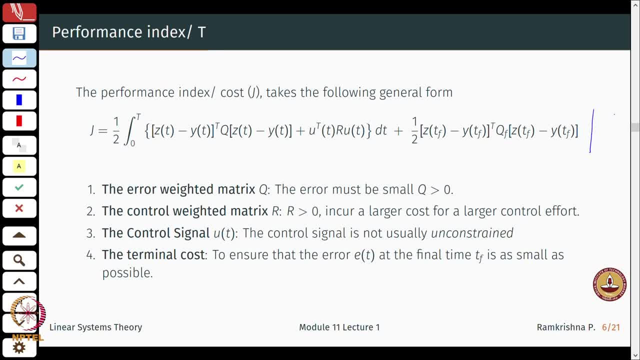 So what are what I am I interested in, right? So what does this entire integral here mean, right? So what is ok of these terms? a little in detail, ok. So first I have some difference here: z minus y, z minus y, something to do with the inputs and something which has some tf here, right? 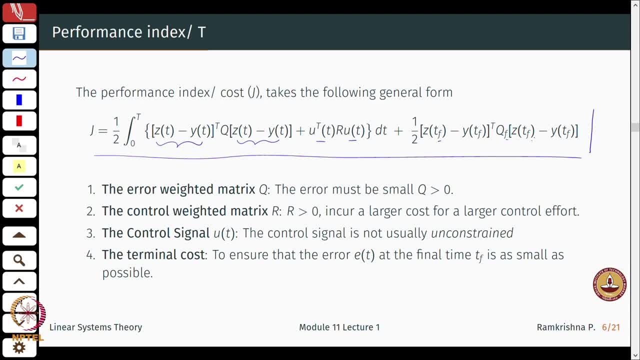 So we will just analyze what are each of these terms. ok, So let me say that the first term in general could correspond to some kind of a tracking error, right? I mean, if I just want to my state to go to 0, then it will just be that I am just looking at x minus 0.. So 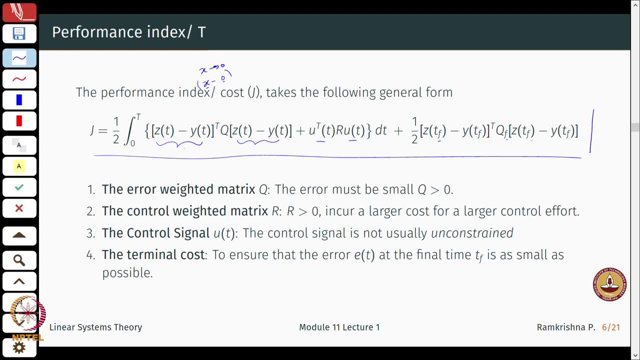 this is my reference, this is my actual, and so on. So this is something to do with the error. ok, Error, some term q here I will tell you what this mean. this is the input. again, some matrix are here. ok, So we will come to this term a little later. 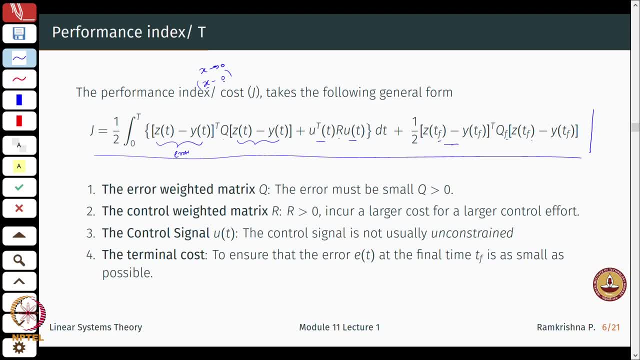 ok, So first, what is the first one? The first is the error weighted matrix q first, is that: well, Usually you would want, or we would want, the error to be small. ok, So this usually has the form e, transpose: ok. So lots of people use also this 1 by 2, just because when you 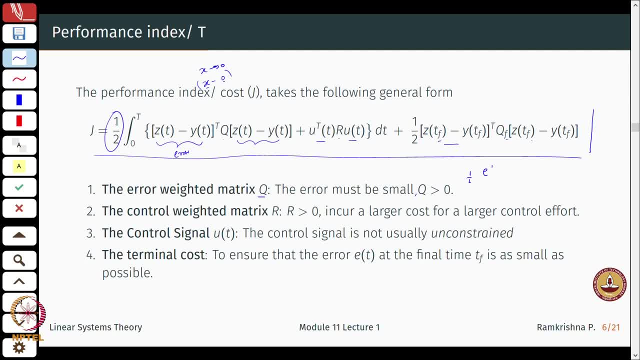 differentiate, the 2 will go away, but without loss of generality you can also remove the 1 by 2.. So I am looking at a signal which is of this form: e transpose t, q, e of q. So I am looking at a signal which is of this form: e of t. ok, Now, typically. so this could. 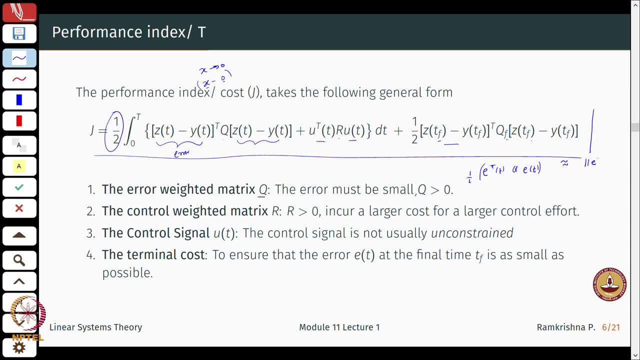 also have some kind of interpretation in terms of the energy of the signal. ok. Now, well, the this should always be non negative, ok, So this is a little approximation. when say q is say identity, for example, ok, This is so. this quantity is always non negative. So 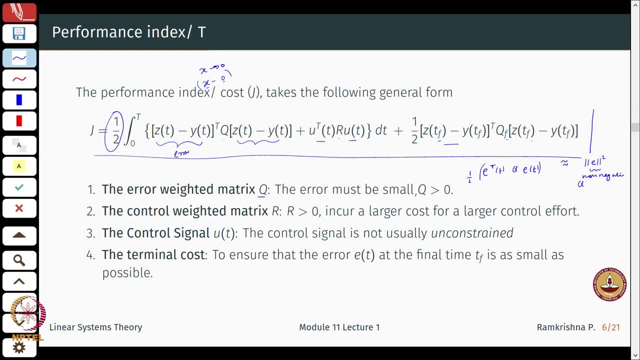 this is a positive definite And therefore the nature of q- and sometimes it could also depend on t- is such that it is positive definite. ok, So what do we have to pay attention to? We may have to pay attention to large errors, and they are not, they are not usually permissible. Now, second thing I have is the control weighted. 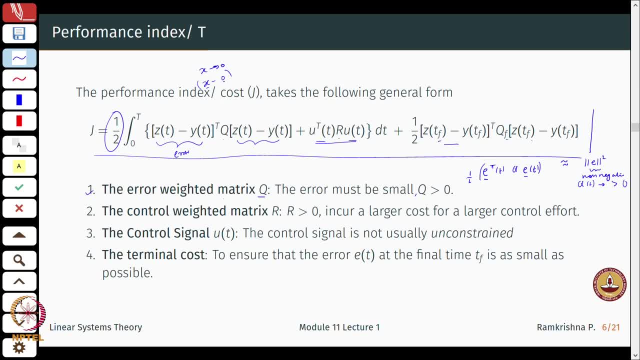 matrix. So what, what? in the first case, what we know is that the error weighted matrix u should be positive, definite, right. So you just get a, some kind of a quantification of the of the error, right? and then that the error should be small, and so on. ok, 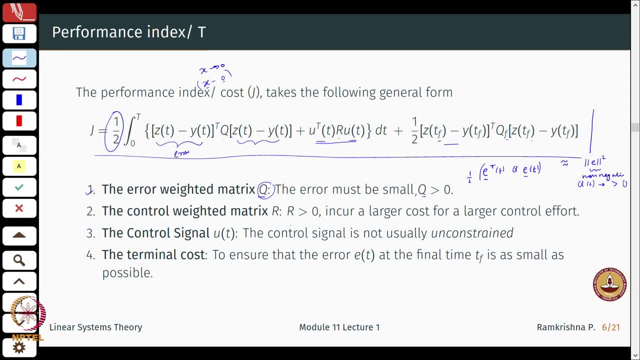 So the control weighted matrix. it also has a form like this: So you have half u transpose r times u ok. So what this means is that well, if r is typically greater than 0, that one has to incur a higher cost for a larger control effort. that is kind of natural right. 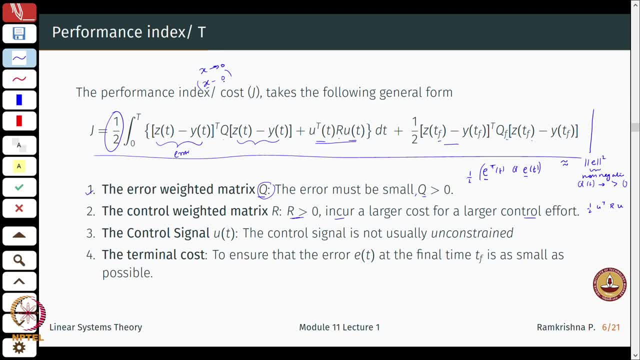 If I want to put in more control effort, I would incur a natural larger cost. say, if I want to have a car which goes, as at say, 250 kilometers an hour, I would possibly not go get that for a price of a of a for Maruti Alto, for example. right, ok, 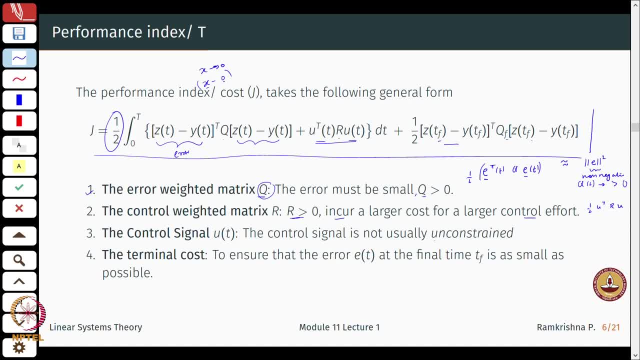 So, and then the control signal? right, the control signal, as I said earlier, is usually unconstrained, even though, while in the, in our basic analysis, we kind of assume that there is a. let us see. well, if there is an unconstrained control, can I actually go from? 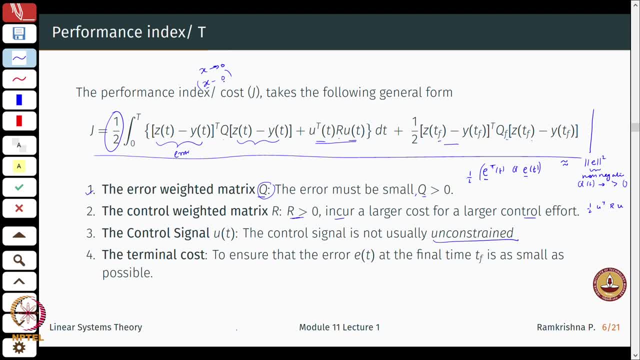 point A to point B. ok, Now what is? what is the conclusion from this three points? The conclusion is that we would like to keep the error small. keep the error small and not pay a lot for control. right, So my error should be small. 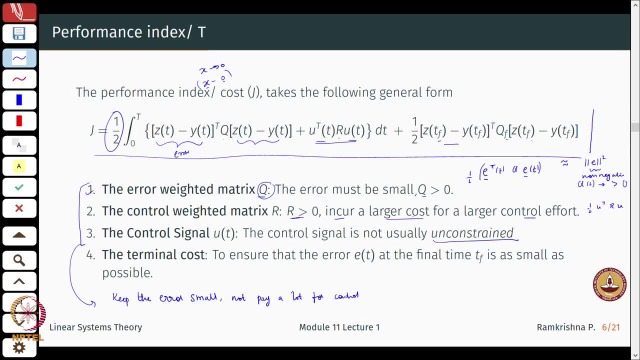 but it should also not incur a large cost on me, ok. And then, last, we have what is called as the, as a terminal cost, so that is taken care of by this term, ok. So the term terminal cost is to ensure that the error at the final time. 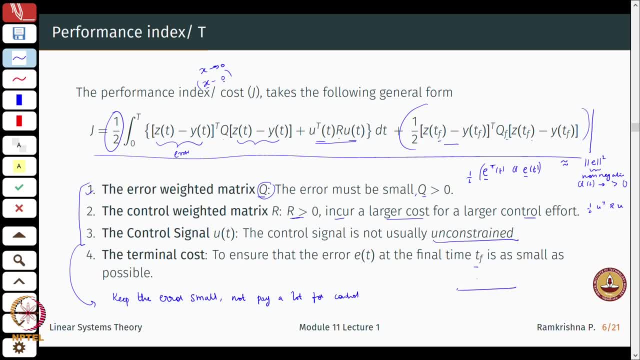 is as small as possible. say, I want to go from point A to point B in some tf, So what? where am I at? at how far am I from the desired performance objectives at the final time is right. So the final time is what this quantifies. ok, And as usual, again, this matrix Q of f should: 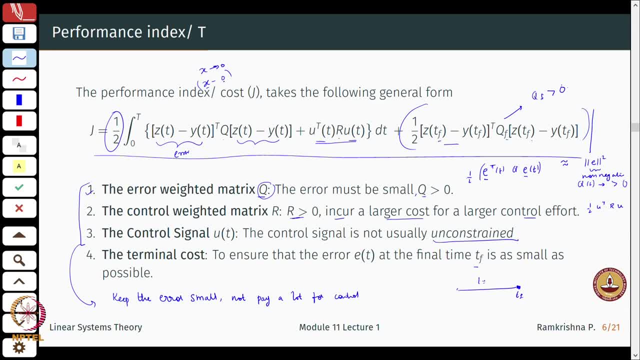 be positive definite, ok. So in general, what I would like to then say- that I want to keep error small, not pay a large cost, and therefore, and at the same time, also have the error at the final time is as small as possible. Now can I design? 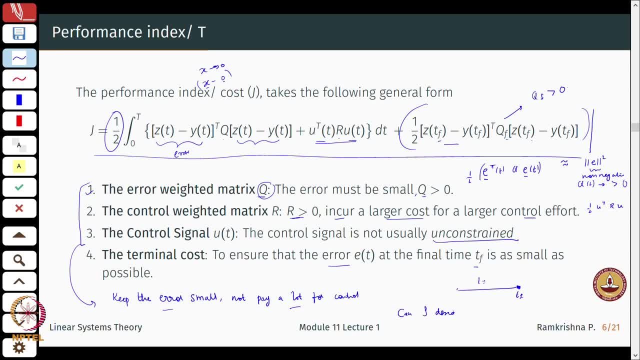 a controller Which achieves these objectives. ok, So again, what my controller look like? controller will just look at you look like this, very similar to what we had previously. Now, what is a good k? ok, Now is there a standard solution to this? 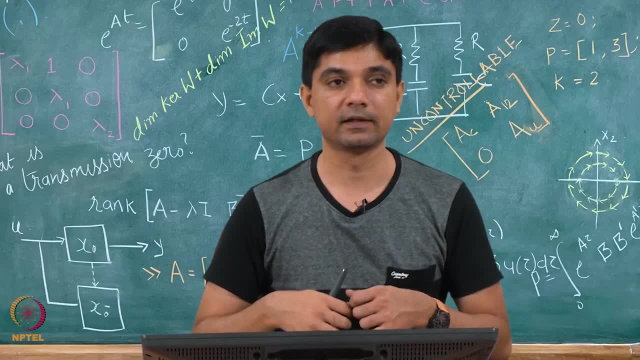 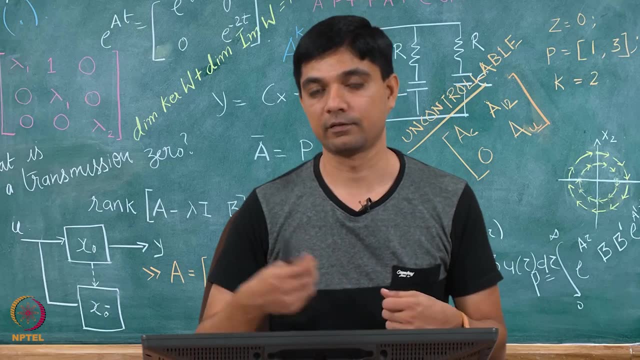 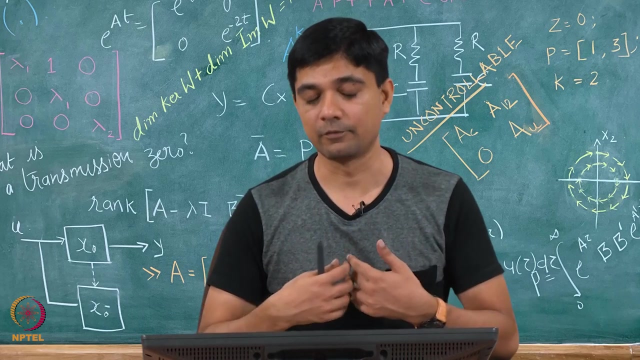 So what will Will be important here is how much importance I give to each of the those quantities. For example, I may want to reach point A, from point A to point B in a shorter time, which means I am willing to pay longer, right? So I am willing to pay a larger amount of money. 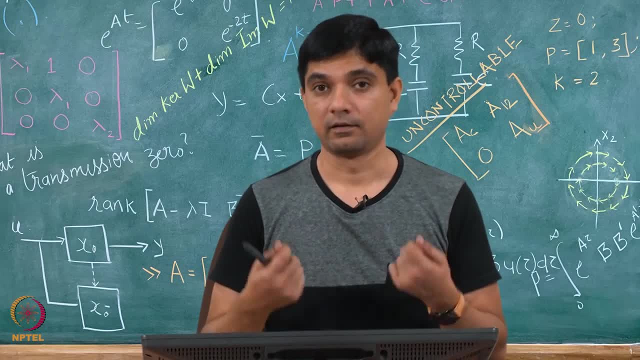 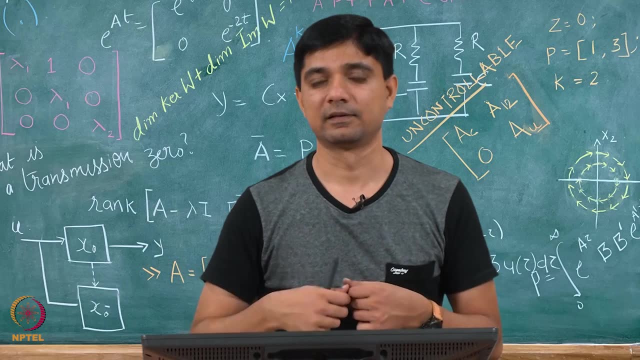 ok, And on the other hand, if I have constraints on on the money of going from point A to point B, I am ok to go by a slow moving transaction. Suppose I want to carry out a public transport or a public transport, for example. right, So 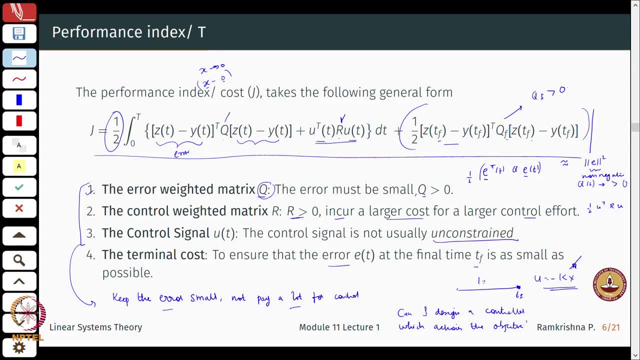 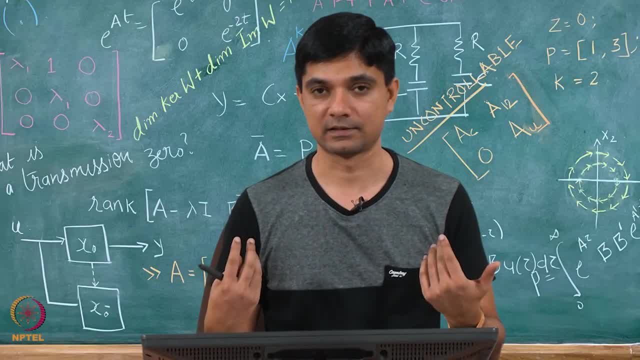 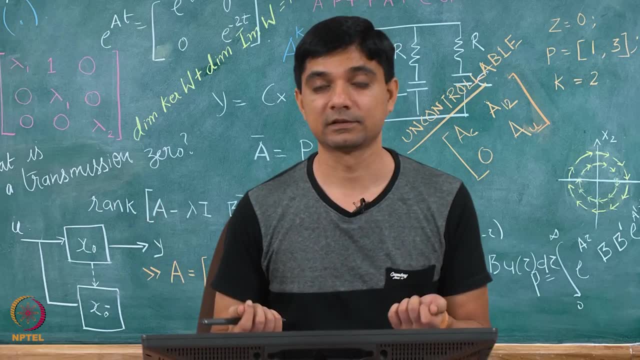 I fix those weights, things via these terms and then decide how am I going to achieve my control objective given those certain constraints. A solution may always not exist, for example, going from Chennai to Delhi in two hours with my little car. It may, it will not exist right. 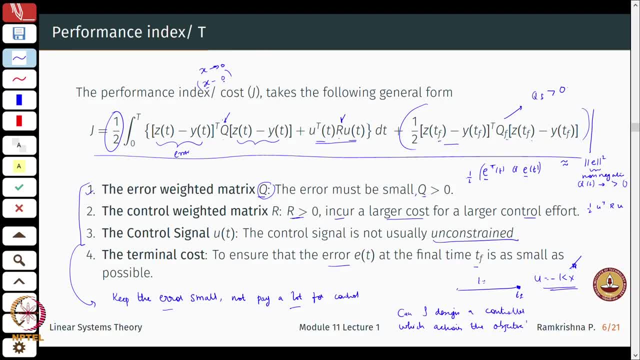 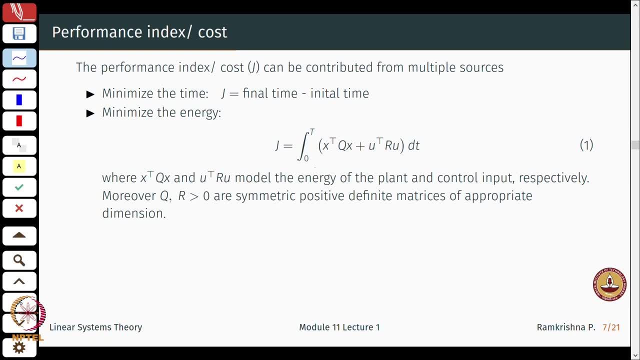 So these are possibilities that we could encounter. ok, most books we will talk of a little simplified cost function in this form right. So we will start just with something which looks like this: right where J is x transpose Q, x, u transpose R, u remains the same as before. So first is, minimize the time. that is also. 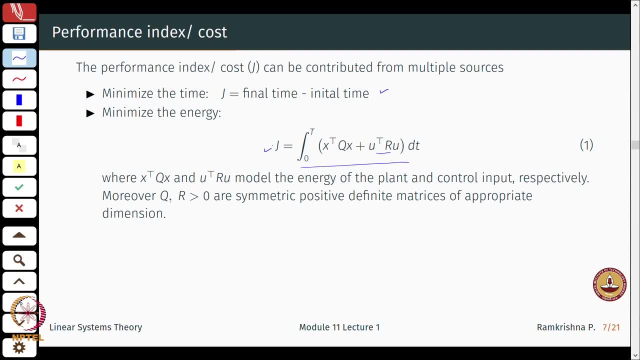 and also, at the same time, minimize the energy right. So, as usual, x transpose Q, x model the energy of the plant, and u transpose u models the control input and so on. right, A little general thing that we at most books. So we are here talking more like, say, a problem. 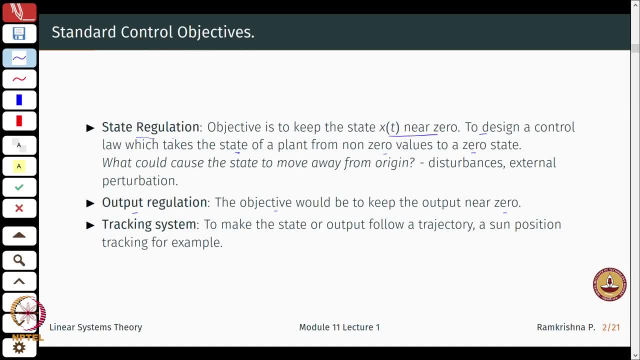 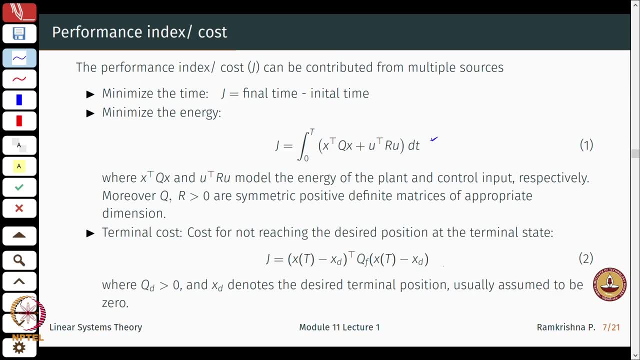 where I am looking at a some kind of a state regulation problem where I just want the states to go to 0, ok, And then, as similarly, I will have some kind of a terminal cost. the cost is the cost of not reaching the desired position at the terminal state and, as usual, I want this to be as close. 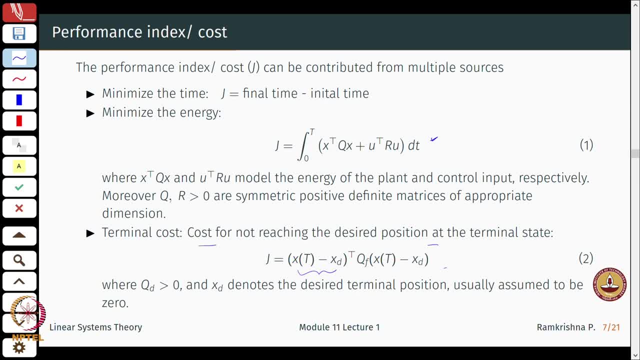 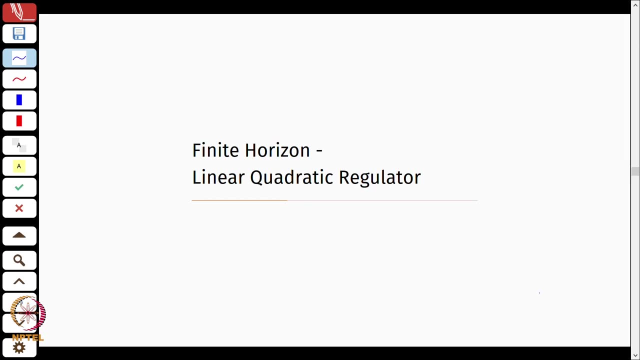 to 0 or x, t to be equal to x desired, at least as closely as possible. ok, So we start with a bit of a assumption that sometimes the terminal cost is assumed to be 0.. So what we start now first is a finite horizon problem where 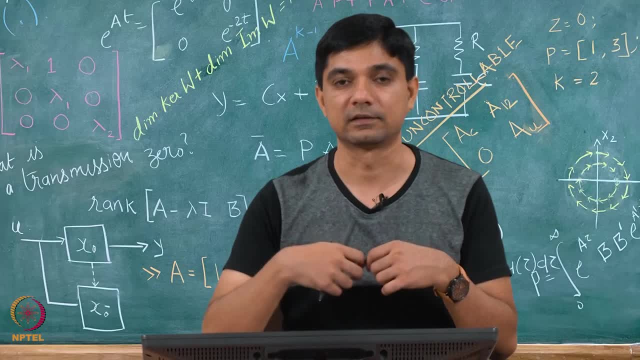 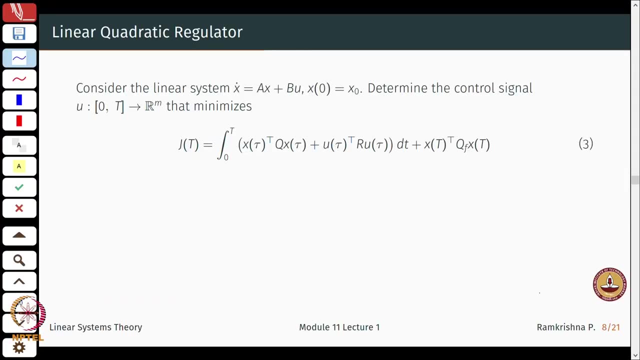 I know that I want to reach from, say, certain initial time and a certain final time is fixed, right, ok, So what is the problem here? The problem is that, given a linear system, x, dot equal to A, x plus B, u, with some initial state, determine the control signal: u. that minimizes. 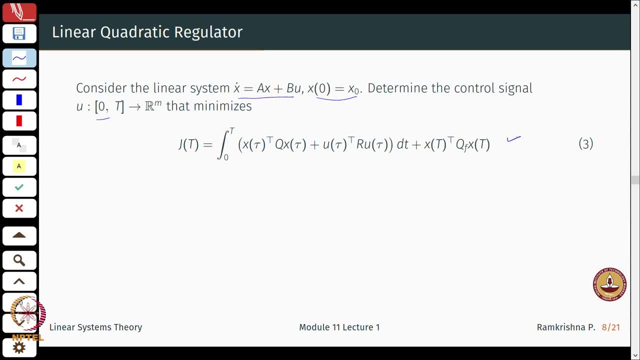 this particular cost function. ok, Now minimize this cost function. So what is the observation here? First is, look, I am looking at 0 to t- finite horizon, problem that. and then I have something which models the state cost, something which models the control cost and something which models the terminal cost. right, 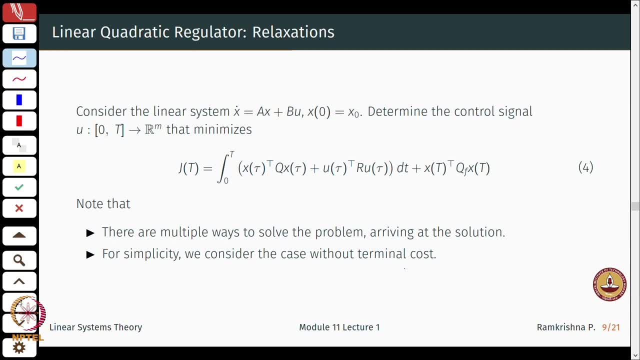 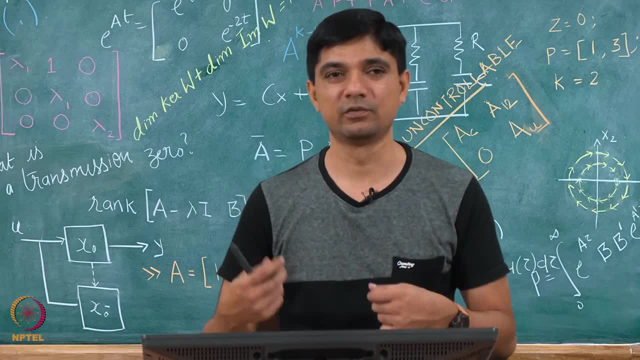 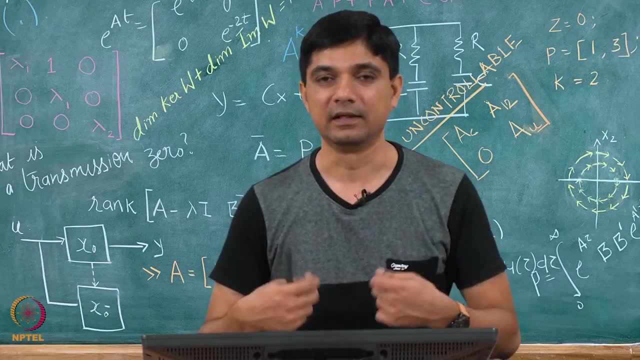 And what we will see, and that there are multiple ways to solve this problem. So I will present you two or three ways which you will regularly encounter in some textbooks. ok, So let us start with that. there might be more ways to that. there are lots of detail analysis, but 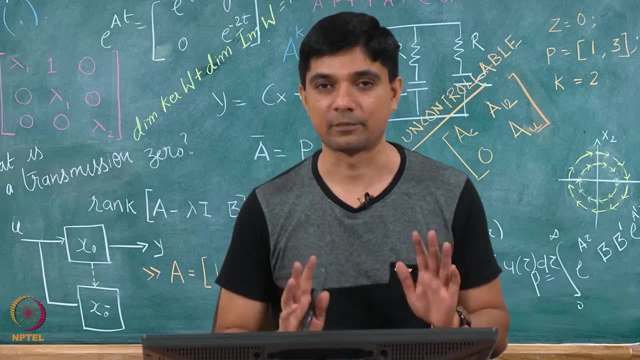 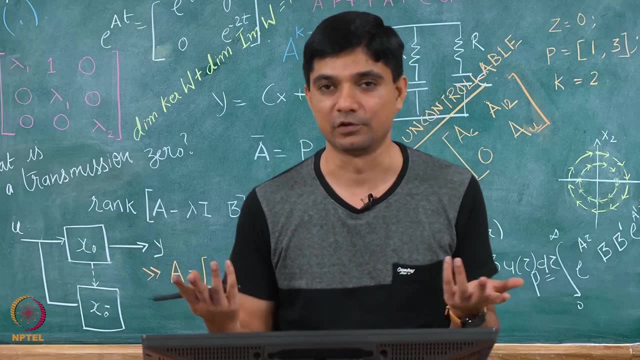 we will try to get for our self a good understanding of what is happening here right through three different methods, and again, you can follow whichever method you want, and all methods give me the same solution, right, ok? So first is, let us start for a case which may possibly. 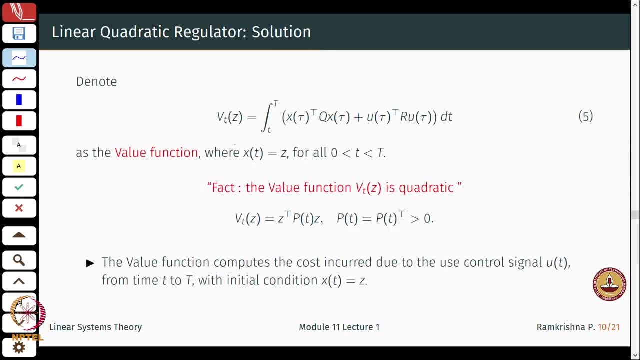 not have a terminal cost. So, which means I have the cost function, which is also sometimes called as the value function. So I have the cost function, which is also sometimes called as the value function, written in this following way: ok, should be here. ok. 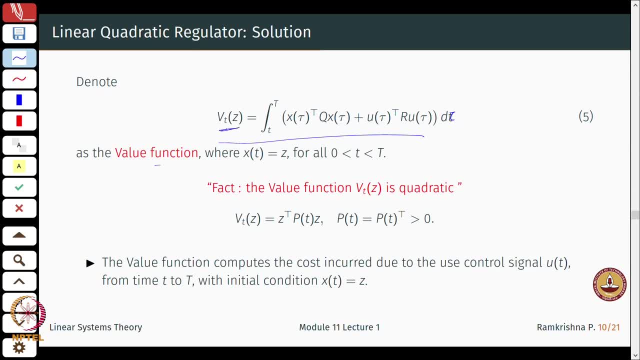 So first is, let me call this my cost function or the value function, right, and let us say: x of t is z for all, t between 0 and capital T. ok, And well, you can see that from here. something which is obvious is that the value function or the cost function is has some. 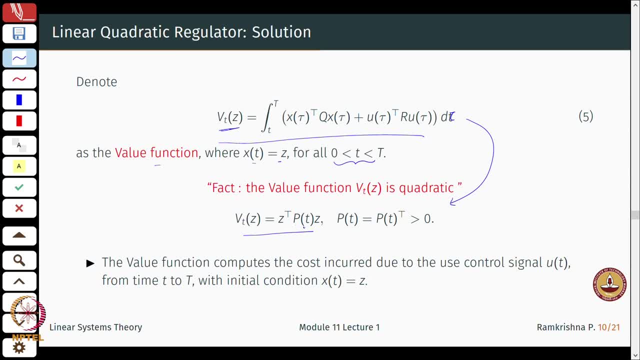 kind of a of a quadrant. So the value function here is a quadratic form: right z, transpose p depending on times, p depending on time t, time z, and this is also symmetric. like this, it is a straight forward computation from here till here. ok, So the value function here computes the cost incurred. 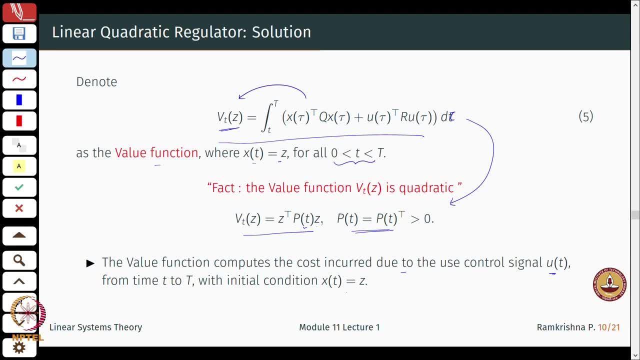 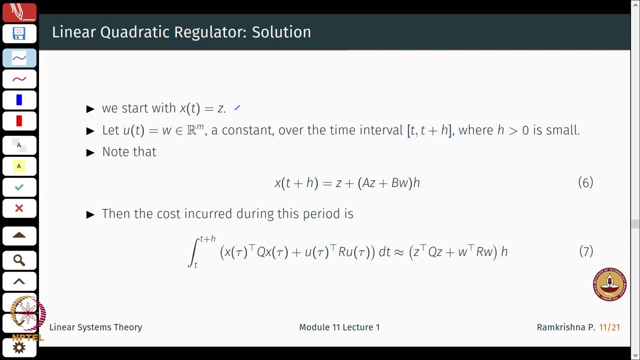 due to the use of the control signal from t to t, with some initial condition given: x t equal to z, right? ok, So we start with x t equal to z, let u t. let me say that that it is. let u t be a constant function over the time interval t to t plus h, with some 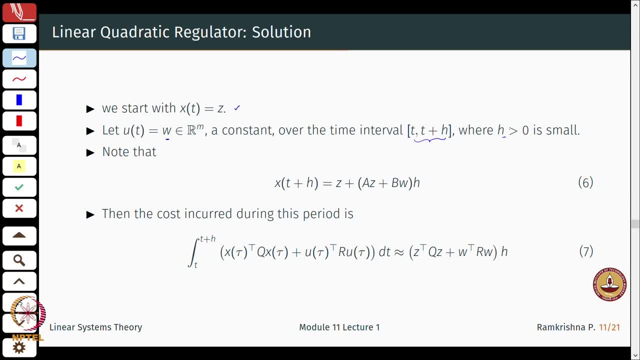 very, very small time: h right. And within this interval I can write x, t plus h in the following way: little Taylor series: expansion right: x t plus h is x dot. sorry, x t plus h, x dot. ok, So this is kind of obvious. and what is what? 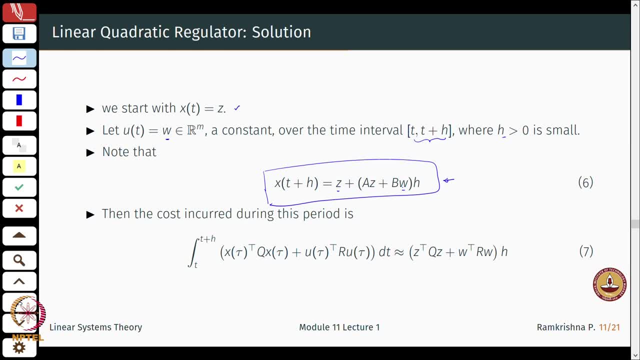 is the state during that time? the state is z and the input is w. ok, What is the cost incurred during that time, or the cost incurred during this period is the following: set x from t to t plus h right x. transpose q again u. transpose r times u, which can be loosely. 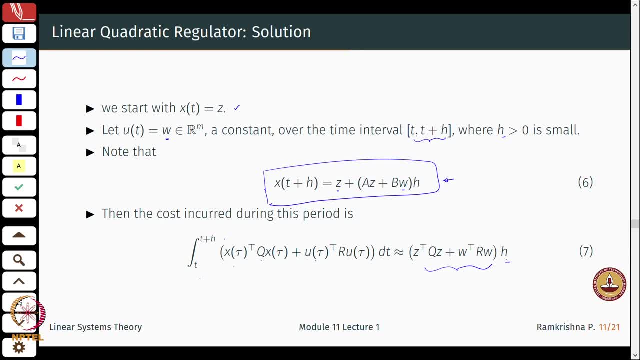 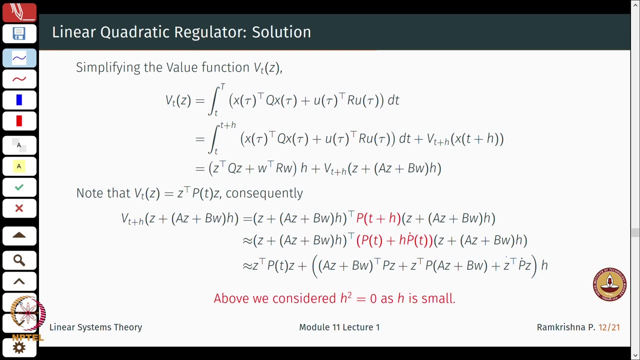 approximated to this. ok, Again, this is just a little time interval from t to t plus h. ok, This should again be like easy to verify. ok, Now, let us see Now. ok, So let us let us, without reading this, steps, let us actually try to try to derive. 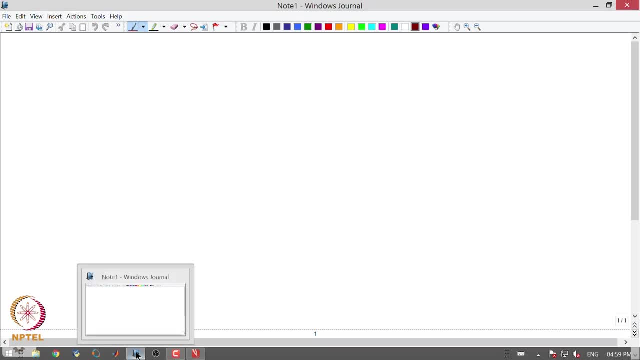 all these things and I will come back to the explanations again. ok, Now, first to simplify the value function v? t of z. So what was v? t of z starting from t to this terminal time? v? t of z. time capital: T x transpose q, x plus u transpose r u t t. ok, this I can write as: 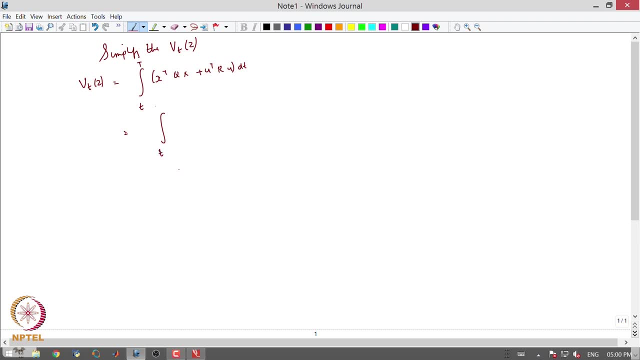 two parts. right one is an integral starting from t to t plus h, with having the same things inside: x transpose q, x, u transpose r, u plus the term integrated from. Now t is integral. Now t is integral. Now t is integral. 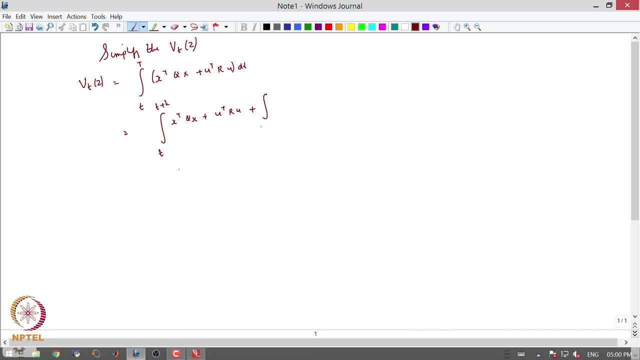 T is integral, now t plus h to t, with the same thing in the bracket. So what will this mean? This will actually be the value function v computed at t plus h, with x at t plus h. ok, So this is just. I am just using the definition of the value function. ok, Now from the from. 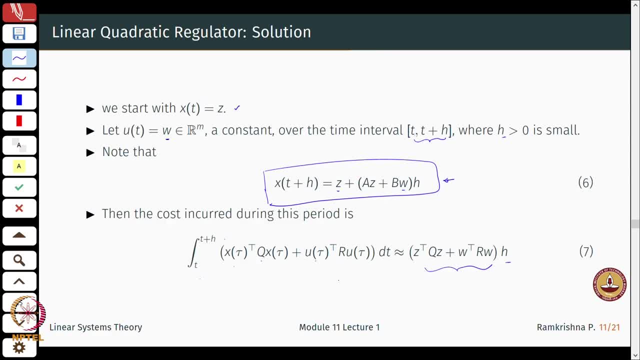 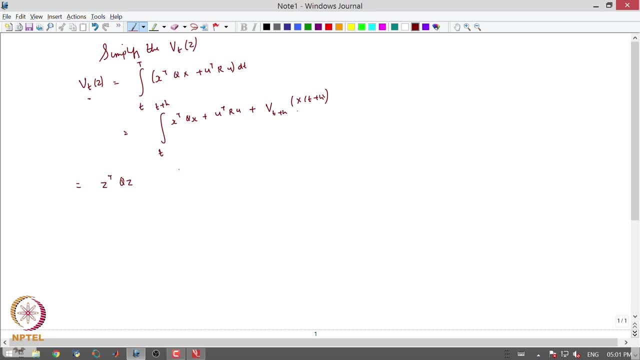 this approximation. here I can rewrite this as: z transpose q, z plus w transpose r w times h plus v, t plus h. Now again go back to this expression right, x, t plus h is a simple expansion. who tell me that this looks something like this: z plus a, z plus b w times h. ok, Now let us see what. 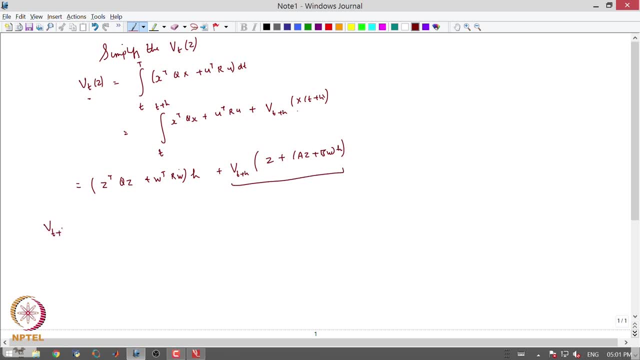 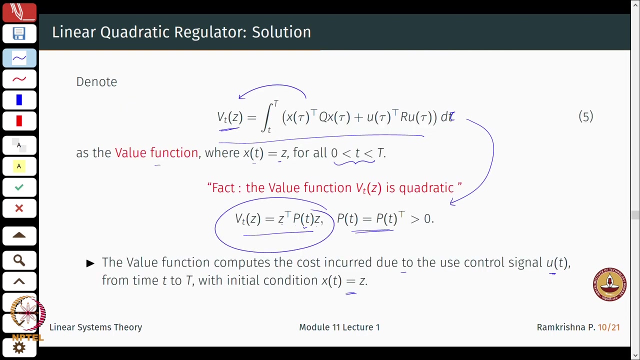 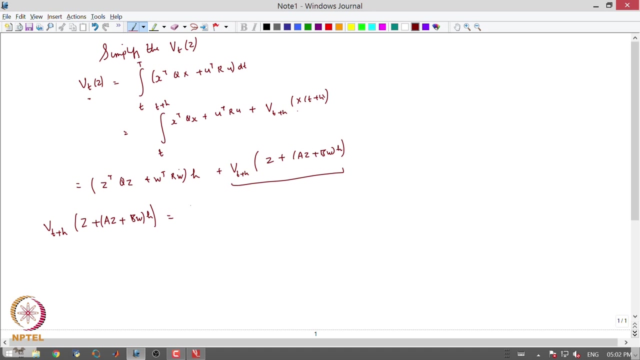 this thing looks like V, t plus h, z plus a. z, Yeah, Z Yeah. z plus BWH is ok. Now what is V like? V is like this: V, t is a quadratic in P and z, So this will be well, z plus Az plus BWH. the transpose P now at P plus H, right? So that is where. 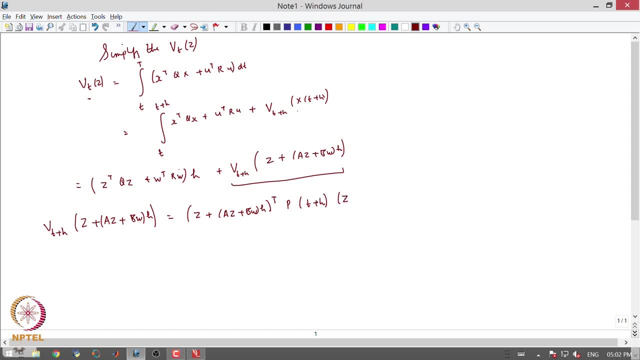 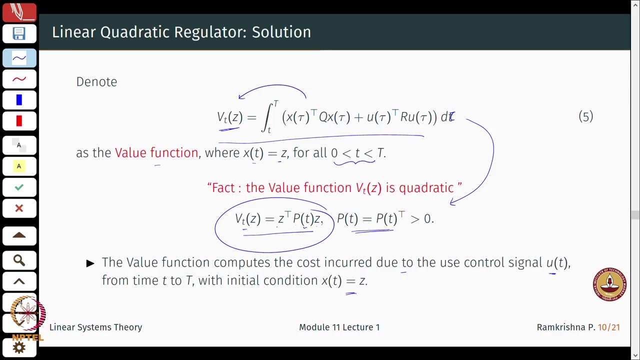 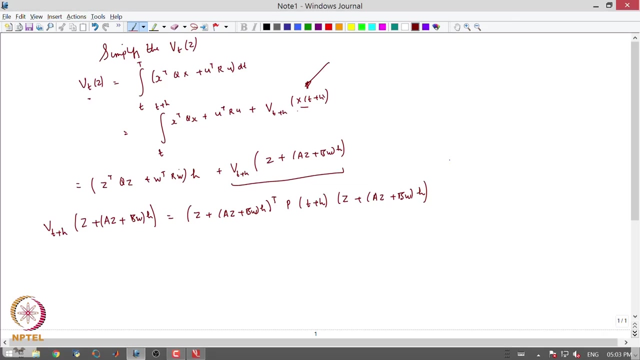 is where we start from right times: z plus Az plus BWH. I am not doing anything special here. I am just writing V, t, right, this for this particular V, with this particular H, where this particular x, where the x is approximated as this function, right, ok, So I will ok. So what is the next step? So, this will remain. 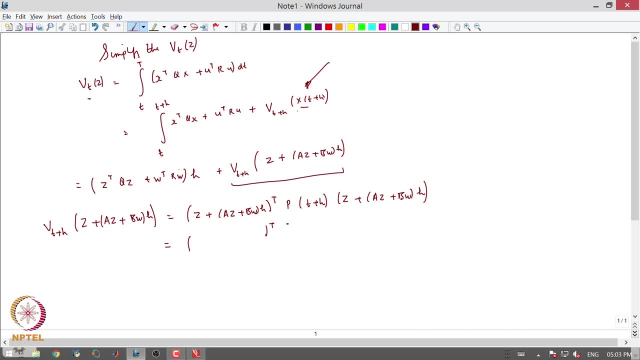 as it is P, I can again further approximate as P of t plus H, times P dot of t, with this guy coming and sitting here again. ok, Now this can be further approximated as z transpose P, z plus H. I will have a bunch of terms here. a sorry: Az plus BW. transpose P z plus z transpose. 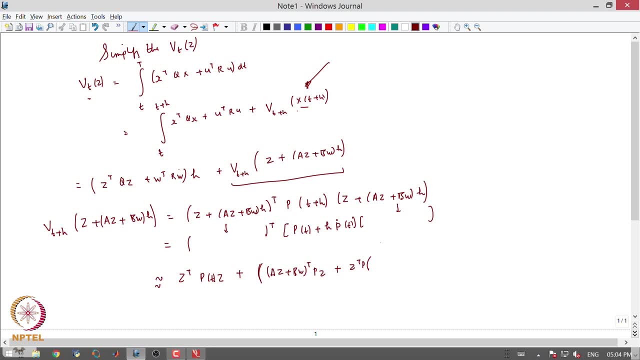 P in P? s are again debating on time: a, z plus BW plus z transpose. I remember some of them. I will explain these here. Yes, etc. I will assume, etc, etc, etc. As I am saying, then I need, we need to read this condition. So I'll have these x and 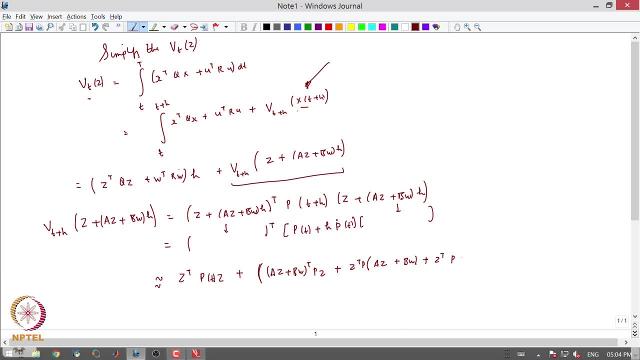 y there for write this term here. ok, Now, what is this? Now, if this, why a plane here z transpose p, p z will be with p dot right. So I am only taking the terms which have a common factor of h, and then you will have something of h square which I will ignore. 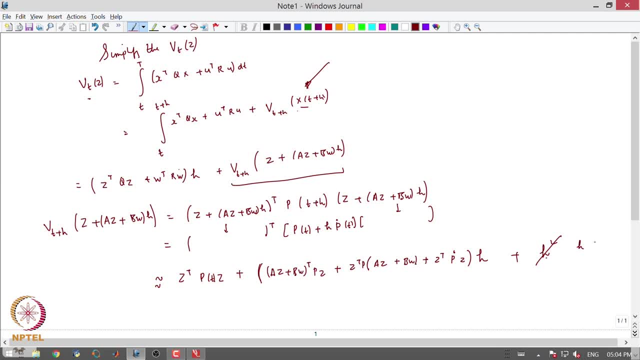 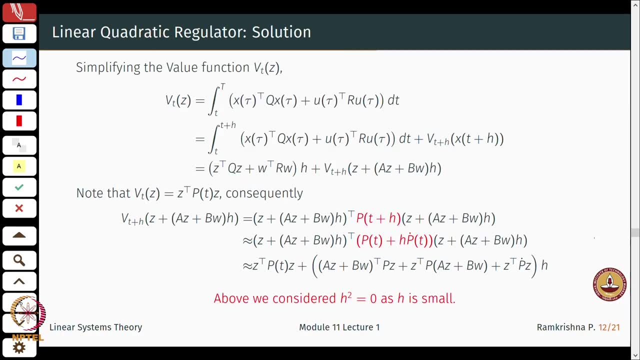 because h is like really small right, So I can ignore these terms. So where are we now? So we started with computing, simplifying the value function. I said I will first integrate from t to t to h and then I have the remaining term over here, which is approximated like: 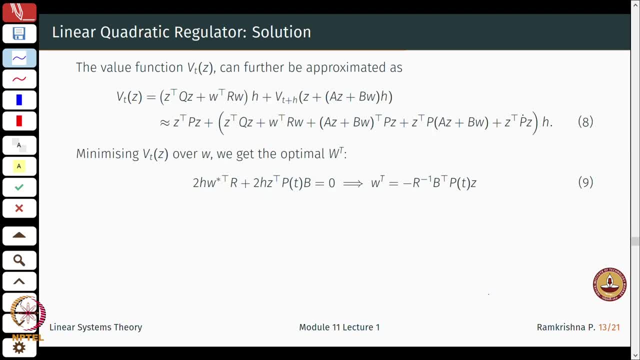 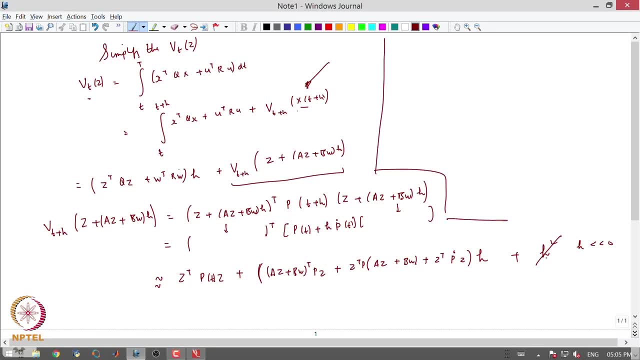 this right. ok, So where do I go from here? So this V t z can now be written in the following way: So the approximation of it. So I am just taking this this term plus what I derived over here, which is equivalent to this: So I will have a bunch. 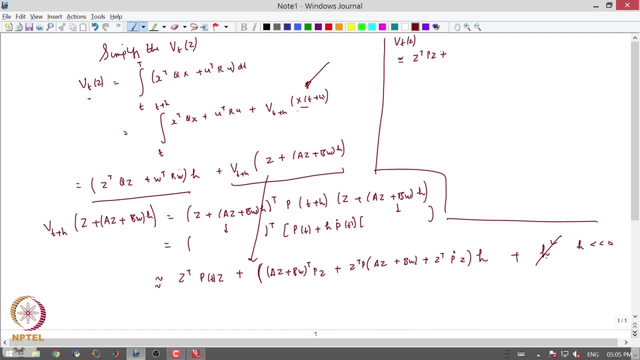 of things here: z transpose P z, plus all the terms with a common factor of h. ok, So there is. So what we will add here is that this term and this term also have a common factor of h. So they will just go here, right. So this term will be as it is: z transpose P z. 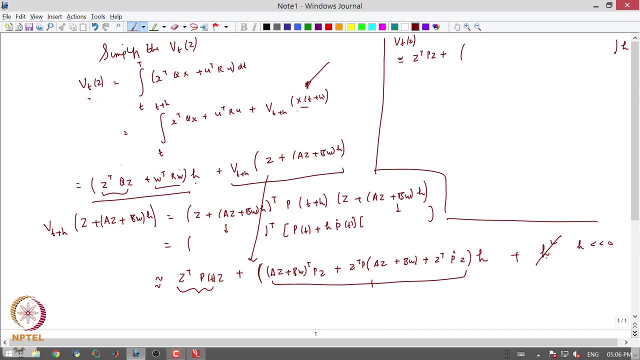 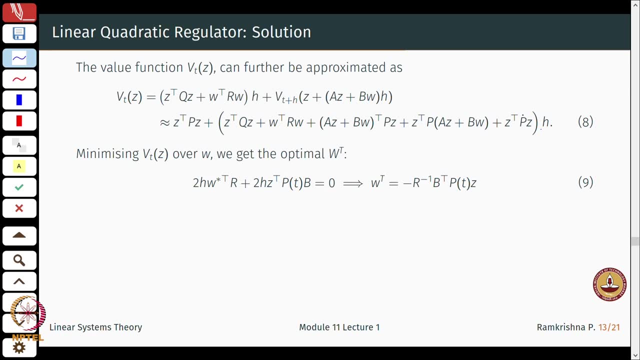 So, whatever is in this big bracket here, we will have two additional terms, this one and this one. ok, So then this is how it will look like. ok, Now what we want to be. So we want to minimize this cost function over what We want to find. 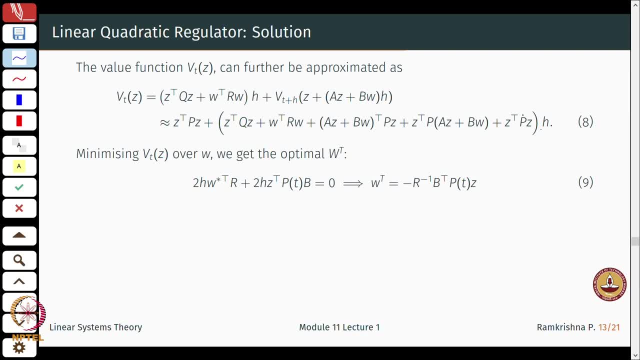 the minimum u. ok, So what is the u here? So I am looking at minimizing it over w, So I get the optimal w, small w. ok, Just a function in one variable which I want to minimize. I just take the derivative equate to 0 and this is what I get, that the 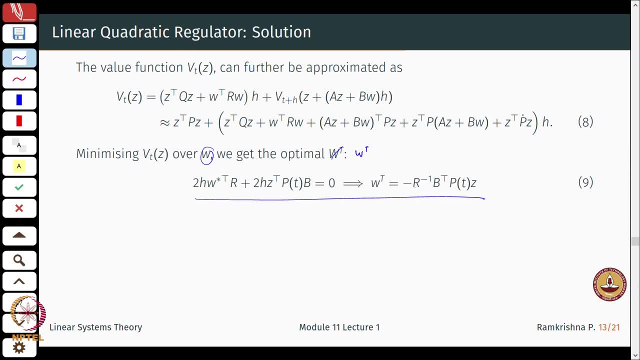 optimal control. w transpose is minus R. inverse B transpose P t times z. Now, what do I have now? So, once I have w, I can now get a state feedback control which is of this form: ok, So what is the w? u is in general right if I look at So for a small w, it look this: 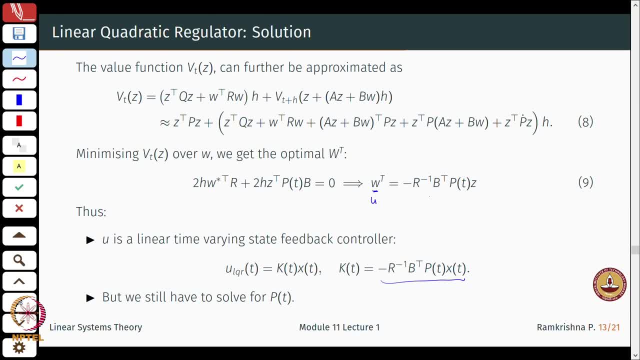 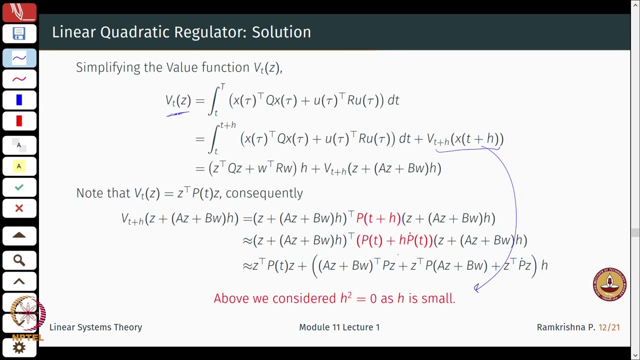 way. So what will a general u look like? This is u, this is minus k, which varies with time times, x, right, ok, Now what do I know from here? I know what is R because I fix the matrices here or I fix the weights of how much, say constraints I have on the input. 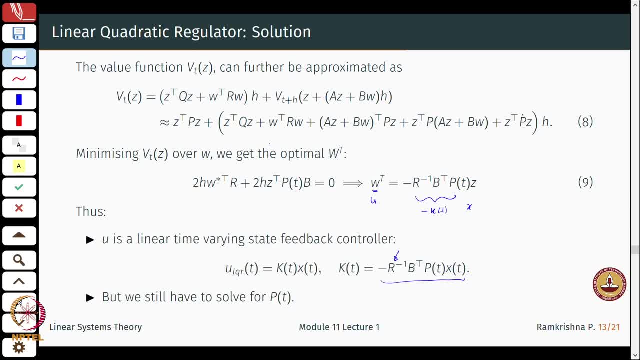 and how much constraints I have possibly on the state. So I know this: P B is given to me. I know x right. So what is unknown here is this term, P. ok, Now to find this optimal input which depends on P via this relation, I still 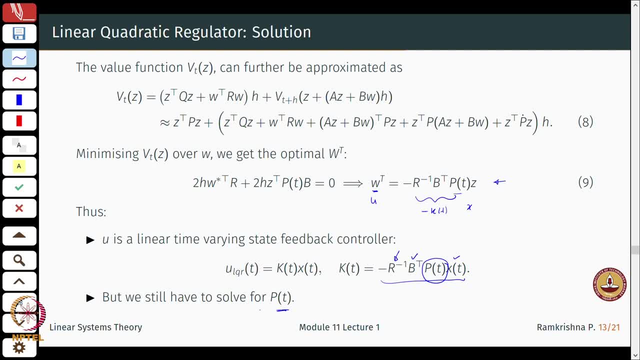 need to solve for this P of t. ok, Now how does this look like? Well, this can be solved by substituting for this: So the u, which was k, x, t, or w, which was this k times z. I can put it back here, ok, So what? 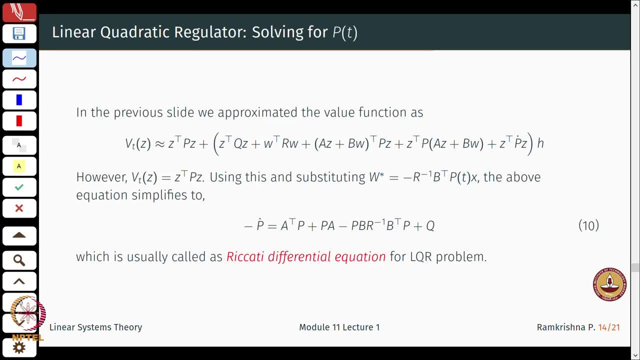 does that give me right? ok, I will just skip the compute, the computations. but what will that give me? that the equation now simplifies to something like this: Now, this is usually called as the Riccati differential equation for the LQR problem. 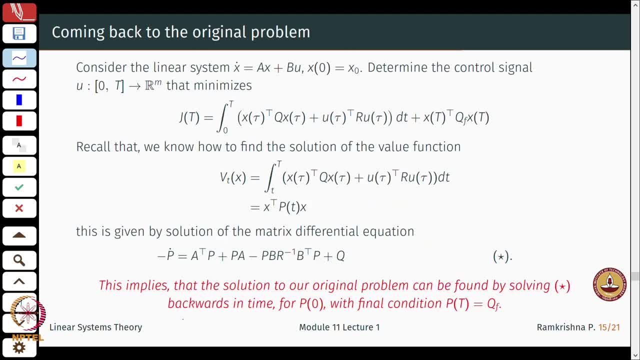 ok, So where did we start off with? We started off by a system dynamics, x dot equal to A, x plus B u, with some initial condition. we wanted to determine a control input that minimizes a certain cost. ok, We know that well. the solution, in the absence of this guy, we know that the solution v, t. 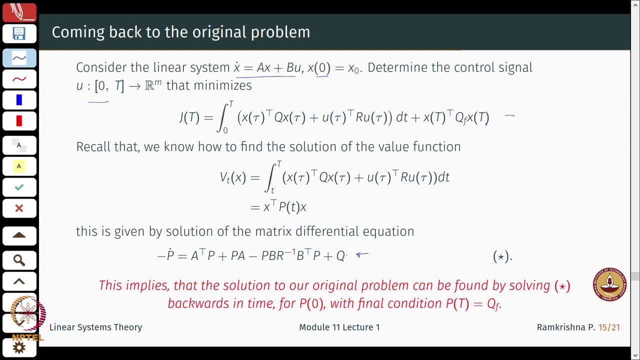 is given by this matrix differential equation. ok, Now this implies that the solution to the original problem can be found by solving for this equation backwards in time for P 0, with final condition P t equal to Q f. right, So that is what we are trying to do. So 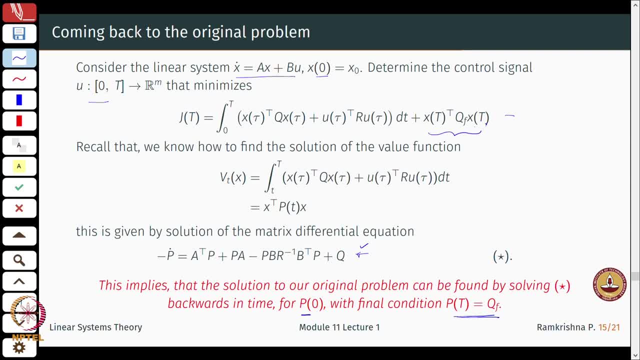 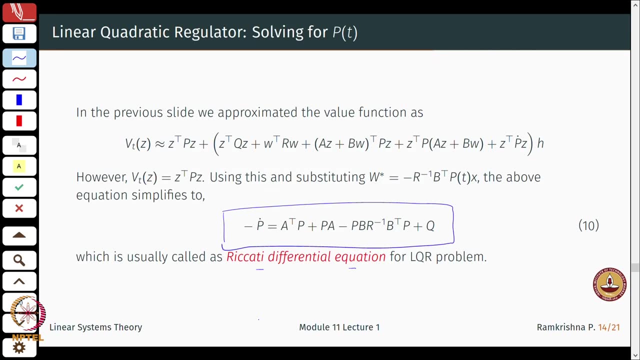 now I can look at what my terminal cost looks like. So I know this P, t is Q, f and I can actually solve for it now backwards in time. So once I know this it becomes a little easy formula. so I can just substitute for that P over here. ok, 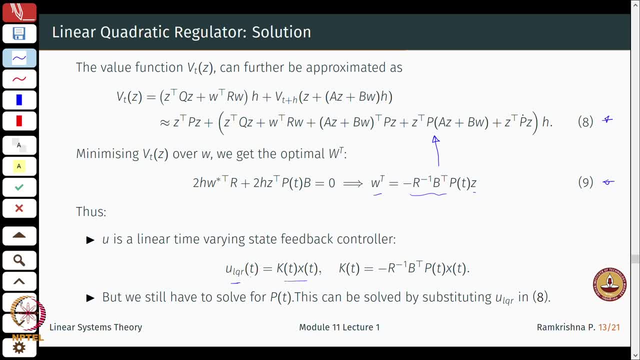 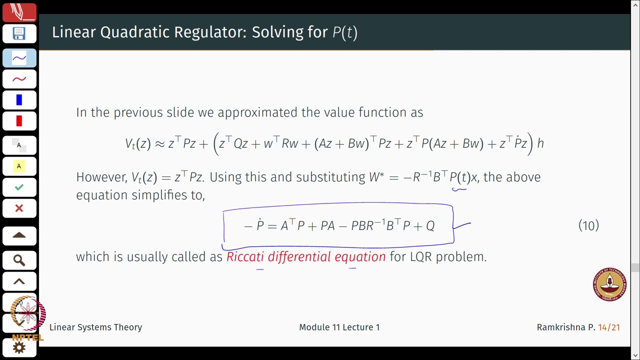 Now this P is again this u of t, which is time varying, will be k of t times x, t and so on. right is that to get this value of k, which is depending on time, I need to solve for this unknown p via this Riccati or via this matrix differential equation right? 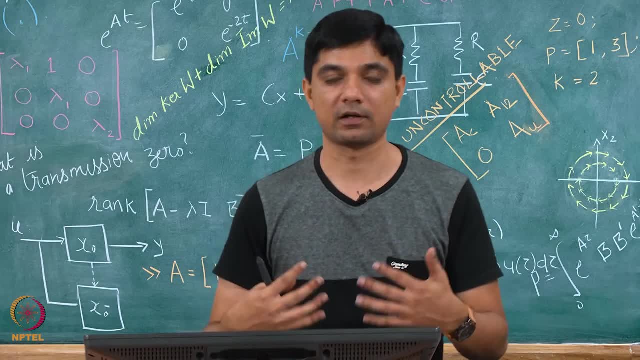 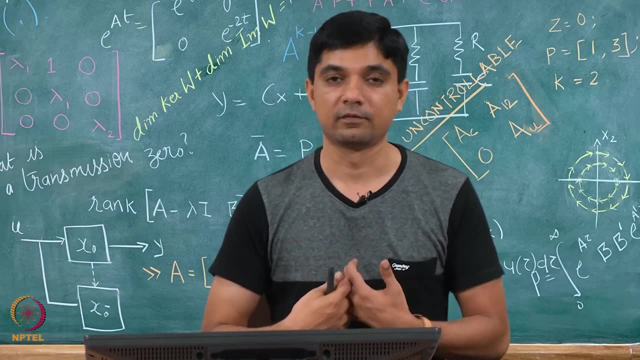 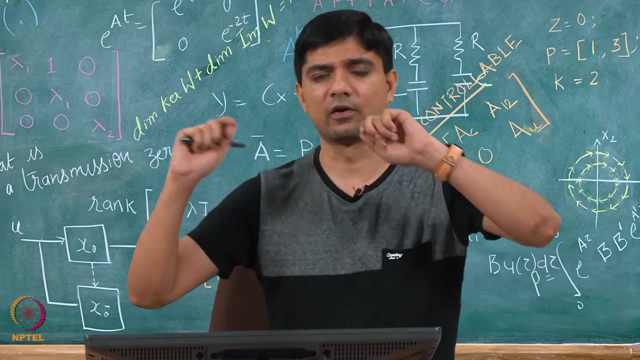 So that is a little basic building block to what we are up to here, right? How do I solve the optimization problem or the optimal control problem? Well, that turns out to be coming from a solution of the matrix differential equation. It is something analogous to the. 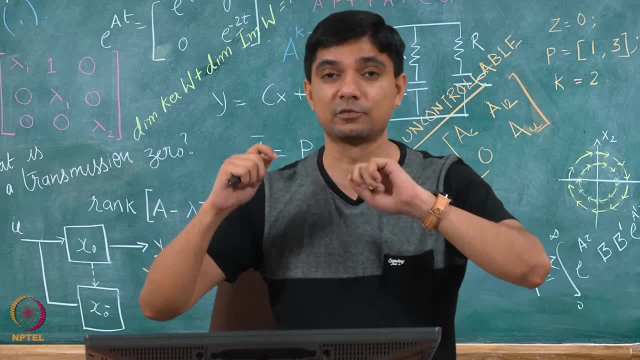 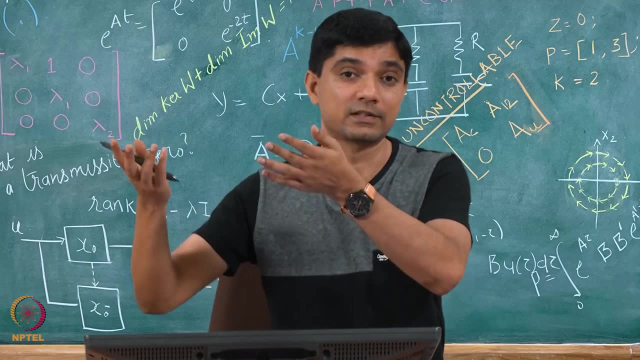 matrix, the Lyapunov matrix equation that we had. A transpose p plus p, A is minus q. but does the solution always exist or not? this depends on whether the system over there was stable or not. It also depend here whether the system is actually controllable or can. 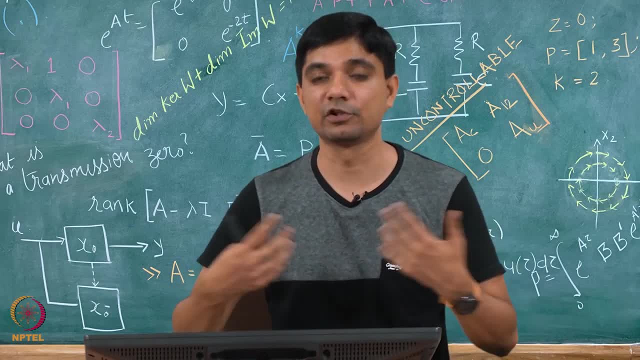 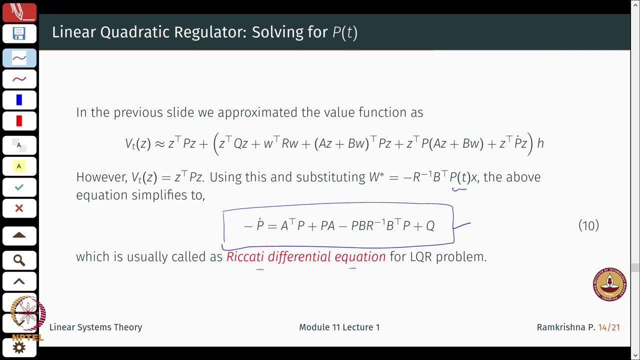 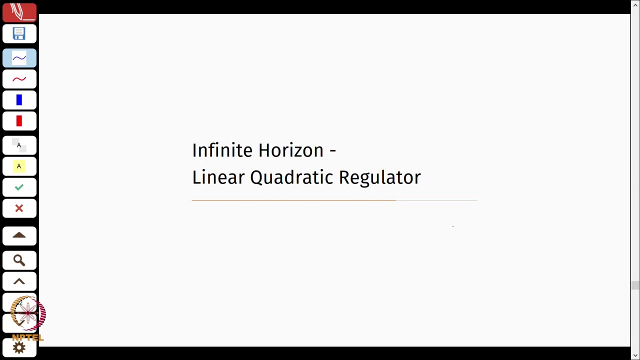 I actually know the solution is not, But not does not always exist, and you possibly will see problems also where the solution may not exist. ok, The next thing, which I mean most books will talk about, is the infinite horizon problem, In a way that what will happen when I am looking at the infinite horizon? 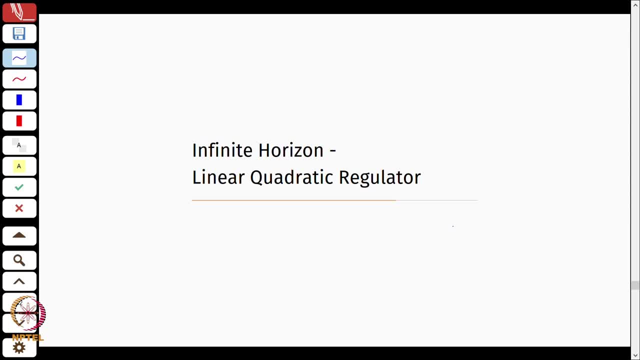 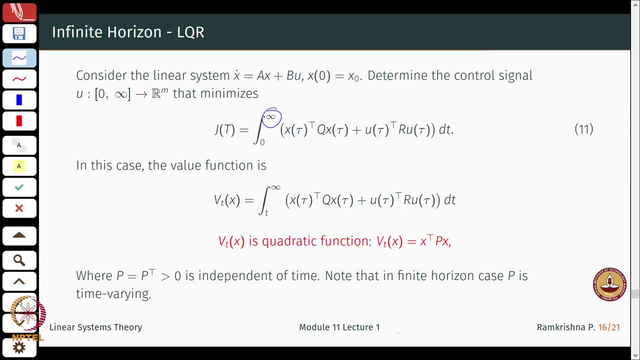 problem is that, well, the final time is infinity, right, So the- this is the case of infinite final time and the tf is infinity, and then the final cos term may not, may. this may not be or may not have any interpretation, may not have any realistic interpretation. So 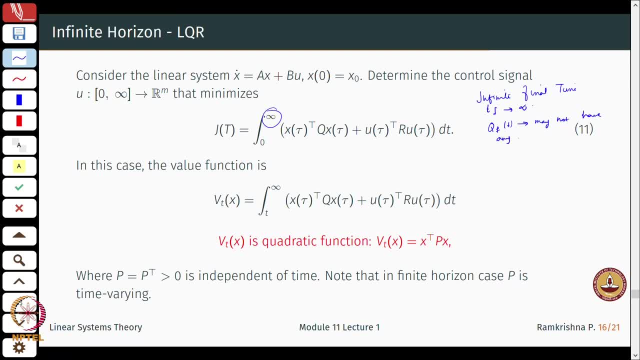 this is the case, OK, Since we are interested, you know, usually in solutions over finite time, and just therefore q, f in this case, must be equal to 0. So we are solving now for the same problem with no final cost and the cost j going from 0 to infinity. ok, So in this case, the value 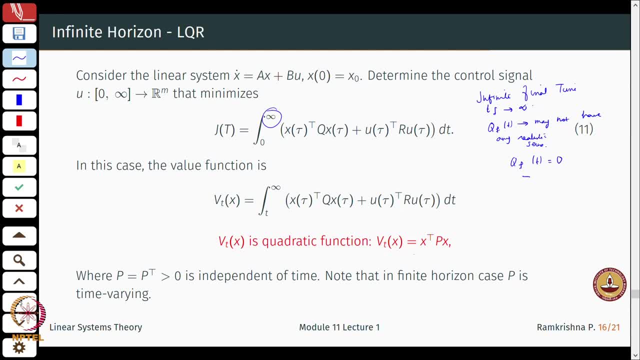 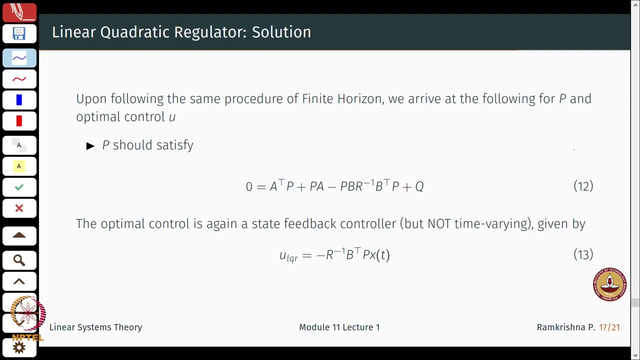 function, or the cost function, is simply quadratic. it will now be independent of time, because, well, there is nothing really associated here. ok, Now the problem now turns out to be to be kind of pretty simple now, So I am just looking now at a solution. So, instead of 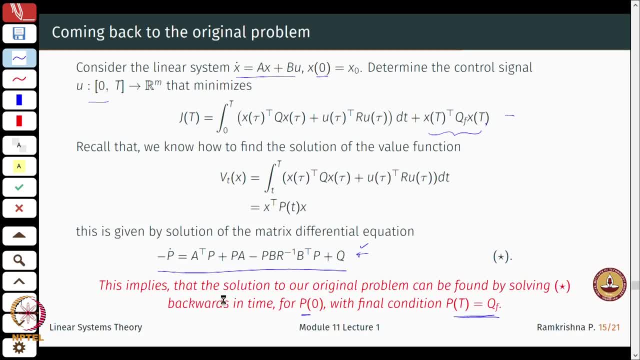 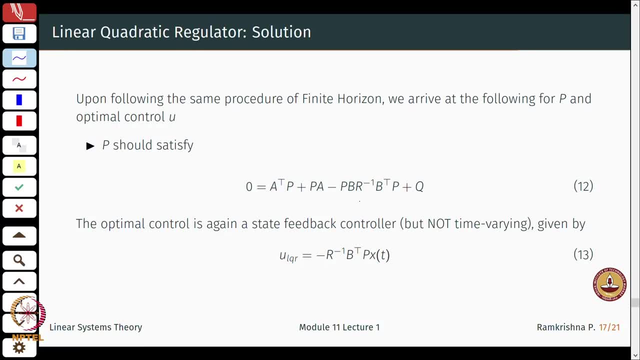 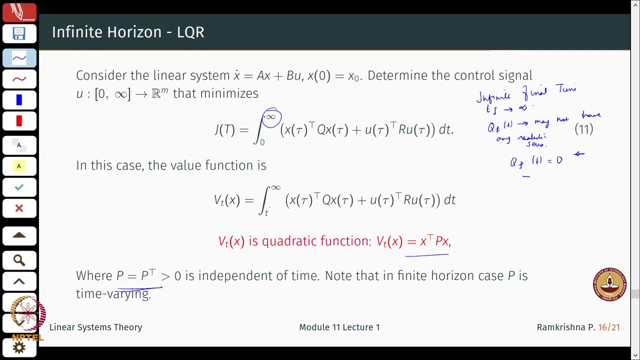 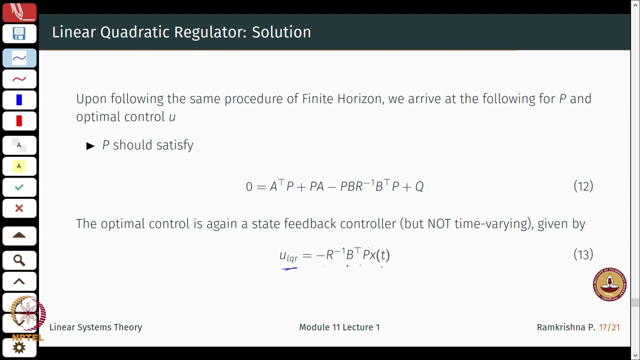 a matrix differential equation. I just have some kind of a linear like looking equation. may may, maybe not right, So I am just having maybe a non-linear equation here. there is no differential term here, So the solution that will give me the optimal control law is minus R, inverse B, transpose P times x, where P is now solution of this. 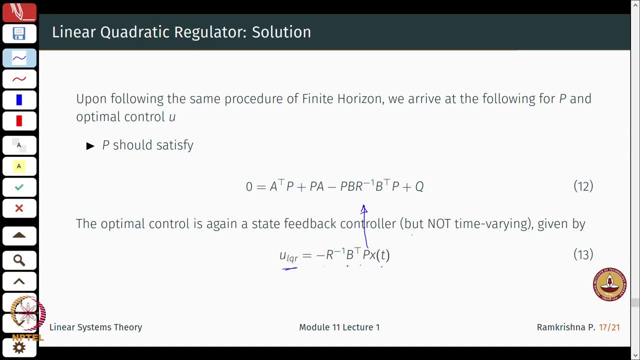 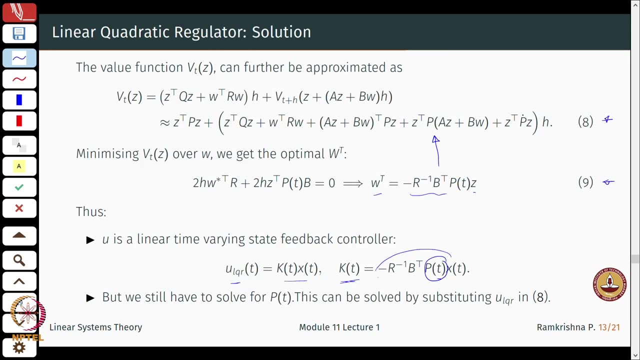 equation number number 12, right. And what is important here to look at is that the state feedback controller, That the gain k here is constant throughout, whereas in the previous case the gain k over here was varying with time because of the dependence of p on time right. So that is a little distinction. 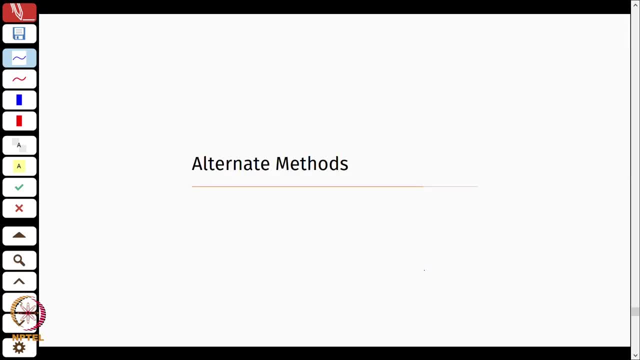 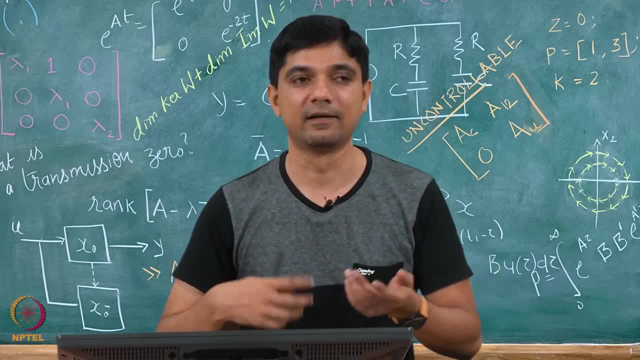 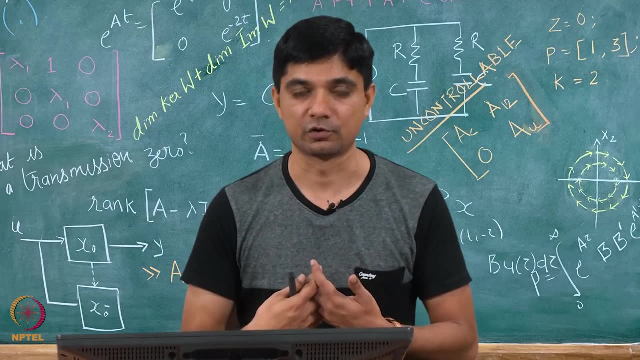 between the infinite horizon problem and ok, So much of the textbooks will first start with the infinite horizon problem. So I just do a little reverse right. So what I did so far was what is also called as the dynamic programming approach. So if you look at Ogata- 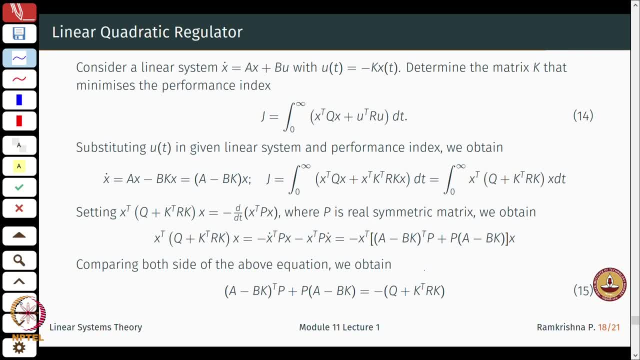 he will have a different method, which I will shortly tell you is in the following way. So consider a linear system: x dot is A x plus B, u, with some input that we need to design and in such a way that the matrix K minimizes this cost function or the performance index. 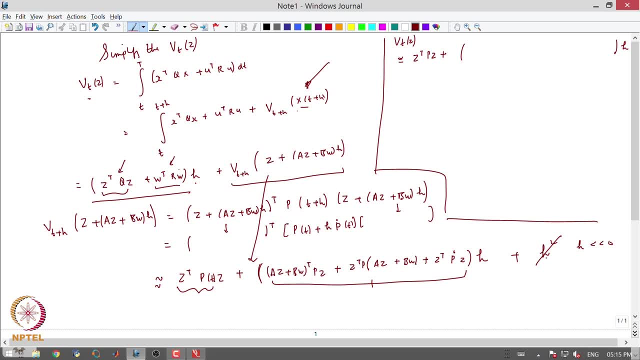 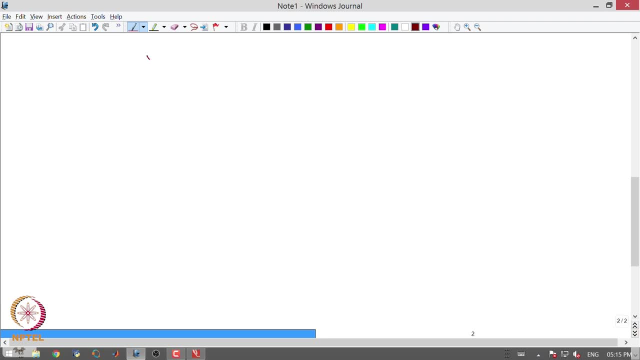 ok, Now what do I know? Let us write down the steps here. So what is given to me is again: x, dot is A x plus B u, and I want to minimize or find a control law- u equal to minus k, x, which minimizes the. 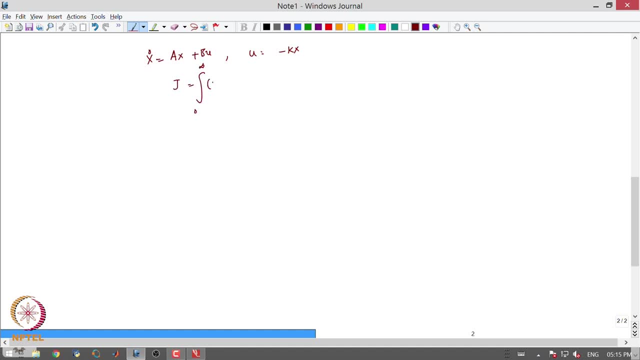 cost functions defined from 0 to infinity: x transpose q, x, u transpose r. you have übers, 이유: x, sinaguang, The u vector and t, that is the cost function. h étant of x, where is constantly a constant? ok, So let me write down the steps here. So what is given to me is again an x dot, is a x plus. 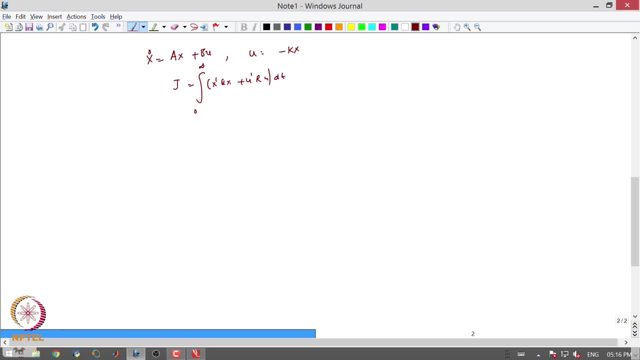 u right. So the times g, t. So this is like the linear quadratic regulator. that is where the name comes from. possibly, ok, So this is the control law, right? and then what I have? what do I have as a closed loop system looks something like this: x dot is A minus B k times. 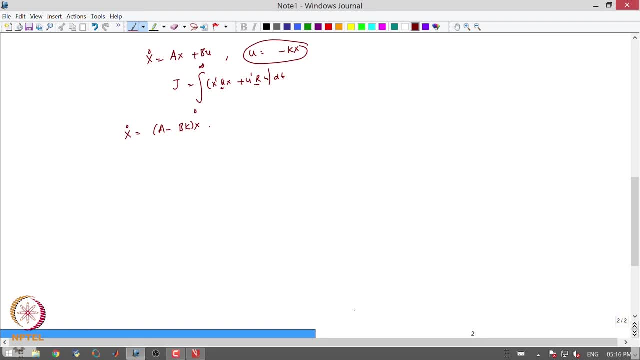 x. right, we have seen this already a lot. ok, Now it will be safe for us to assume that this is stable, right, as there is no point designing this controller. So let us assume that A minus B, k is a stability matrix. ok, And therefore the cost function. now j looks. 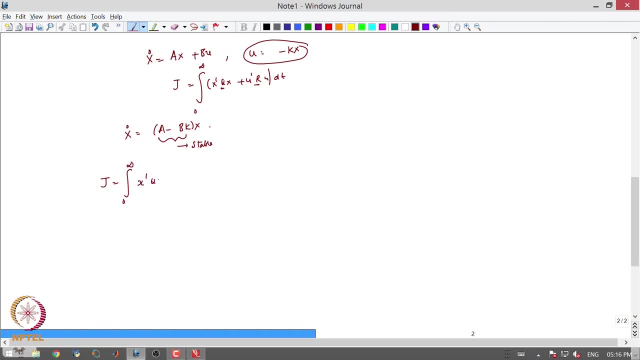 like this: x transpose q, x. ok, So x, this also means transpose, this also means transpose. So this is x transpose q, x plus u is k, x. So I will have x, x transpose, k transpose r, k times x, d, t, ok. So this is of the form 0 to infinity: x transpose. 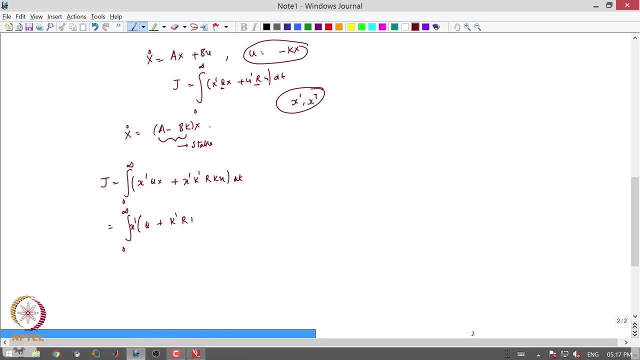 q plus k. transpose r k, x, d t. ok, Now let us do some tricks here, right? So let us set this number: x transpose q plus k. transpose r k times x is minus d over d t. x transpose p x. ok, Now. ok. So what do we know, right? So this x transpose q plus k r k times x. 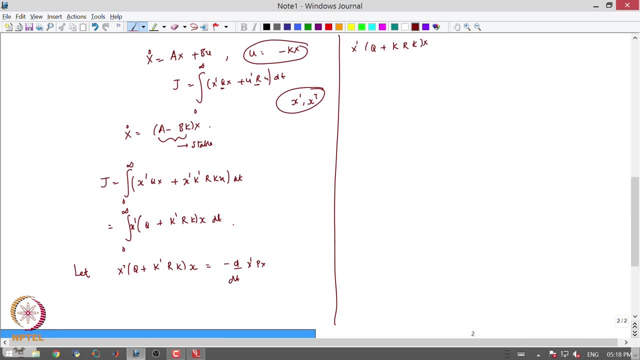 Right, Right, Right. So this x is just differentiate this and get the following: So this is: minus x dot, transpose p x. minus x x transpose p x dot. sorry, x dot here. And this will look like this: minus x transpose A. minus B k p. 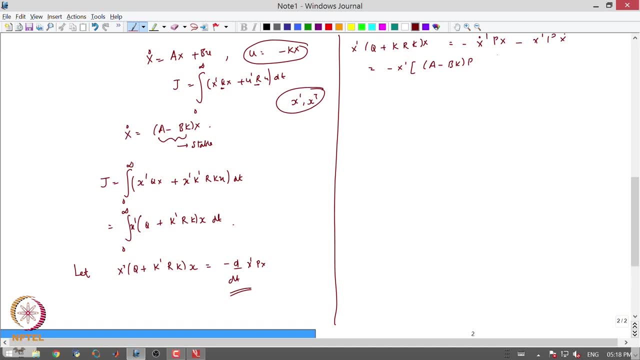 Right B k, p plus p, A minus B k, with a transpose here. ok, So this is something what we had also for the Lyapunov equation. right Now, what do I know? that A minus B k is stable, right And therefore, given a matrix q plus k, transpose r k. 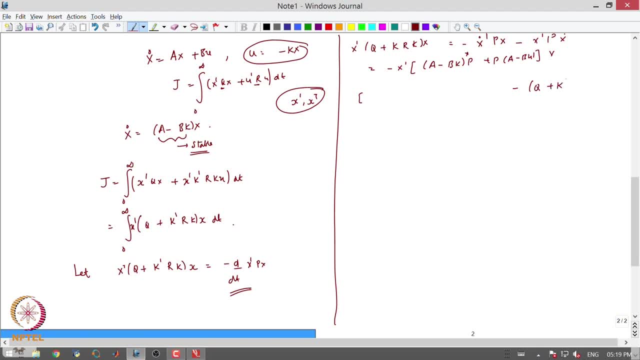 Right, Right, Right Right Now. this is because q and r are greater than 0. this is also greater than 0 for this q. well, I should be able to find a p such that A minus B k transpose p plus p, A minus B k, So some. 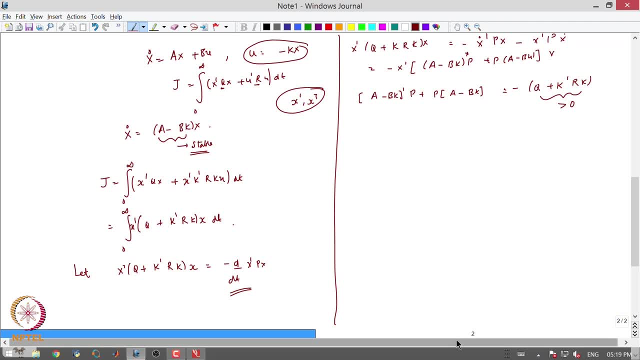 equation, some Lyapunov equation like this holds: ok. Ok Now what is to be found out here, while minimizing the cost function is: does there exist a p which satisfies the solution given a certain optimal k? ok, Now how to evaluate. what is the what? 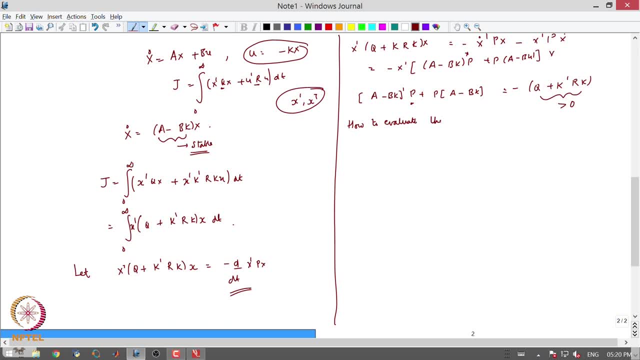 is what is the p or what is the appropriate input, Right, Right. So j, here is now 0 to infinity. now, from here, right, I just do a substitution. So j was x transpose q plus k transpose r, k times x, d. t was x transpose p x: 0 to infinity, right. 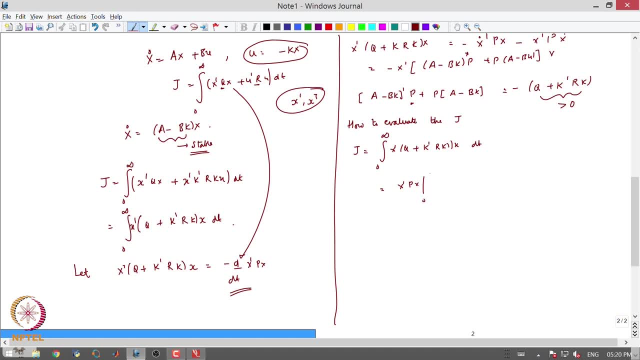 Right Right, Right, Right. So this is x at infinity. this is x at infinity. it will be a little minus sign here because of the minus here. minus x transpose infinity p, x at infinity, plus x, 0, p x, 0. ok Now, since 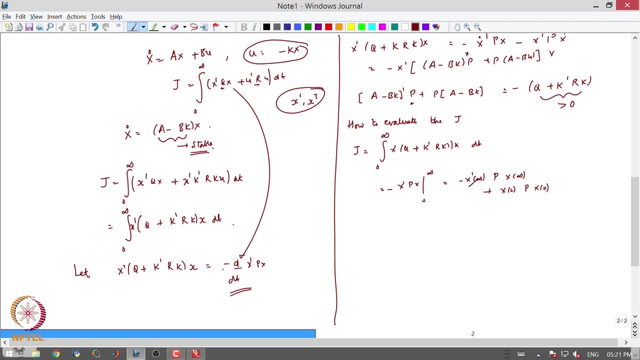 A minus B k is stable, this will go to 0.. Right Right, Right Right. So the next step is z. j is sorry. x transpose p x 0. ok, So this means that I can find the performance index j in terms of the initial condition x naught, which is given to me, and. 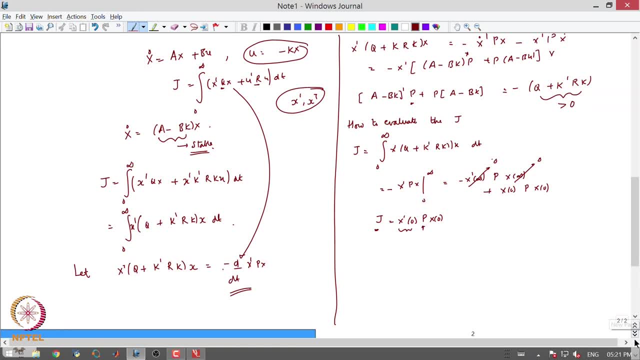 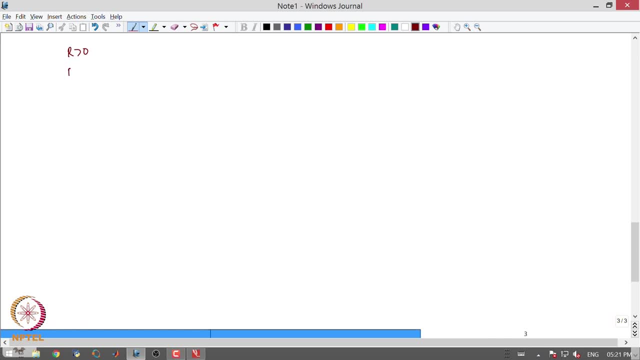 p. ok, Now the next step to the solution is the following: Now, because r is greater than 0, one can always write r as T transpose T. Now I get T, is is non singular matrix and so on, and therefore I can write down my Lyapunov kind. 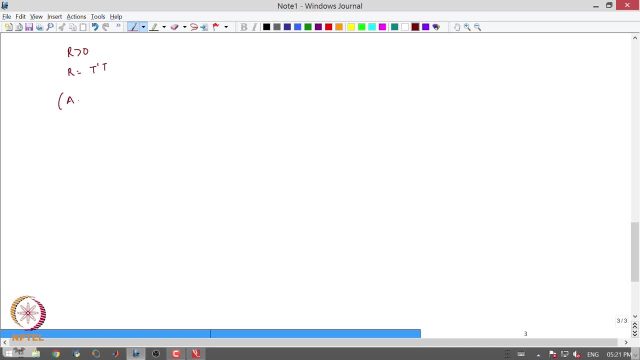 of equation which is like this: right A minus B k transpose p plus P. A minus B k transpose t. Okay, Right, Ok, Ok, Ok, Ok. plus q plus k transpose T. transpose T. T k equal to 0. where does this come from? So? 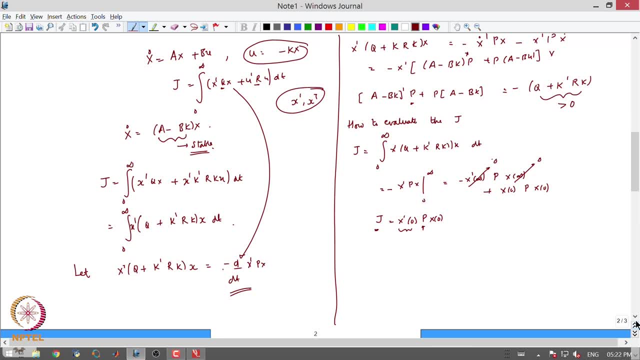 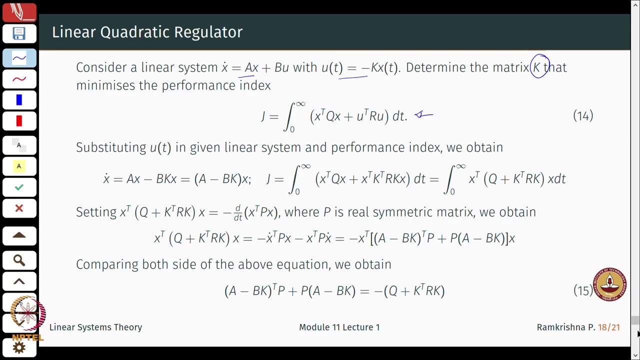 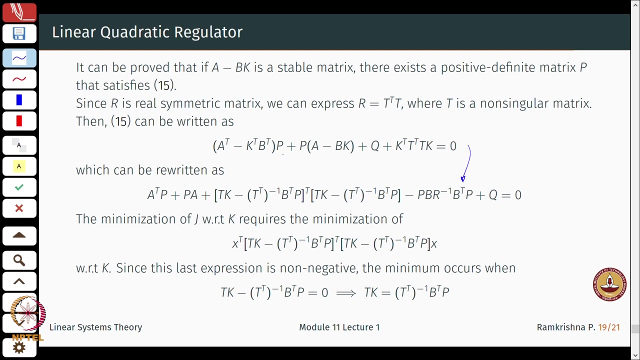 there is a. where is that happening here? So for r I just substitute r equal to T, T transpose: ok. So next, what do I do? is I just write down from here till here, right, I am just expanding terms and minimization of these terms. right again, with respect to k, right? So this is: 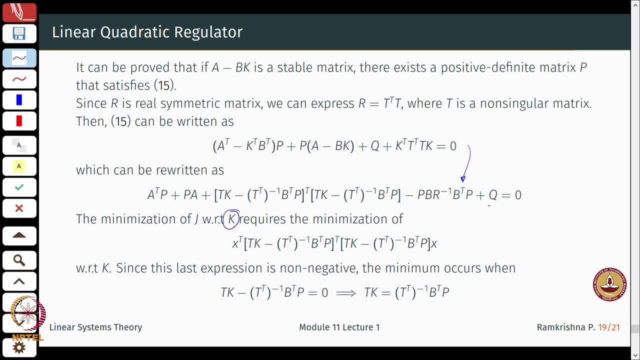 what I am finding. what is a, what is a good k? this requires that this particular quantity be the minimum. ok, Since the last expression, or the last expression, so once we have. So the minimization of j with respect to k, which means we may have 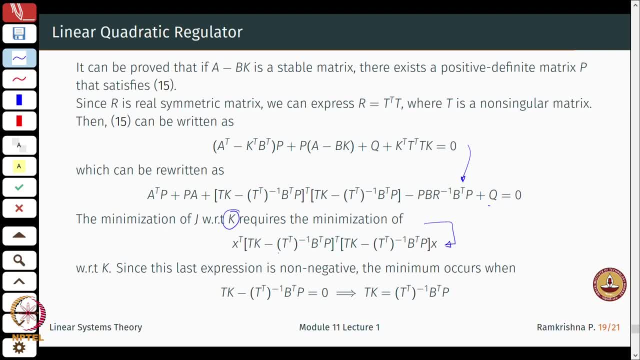 to minimize this term, and this occurs only when look at this right. So I have x- transpose, I have something here with the transpose, something here and x- ok. So this is possible if, and only if, This term here goes to 0, and because this expression in general will be non negative. 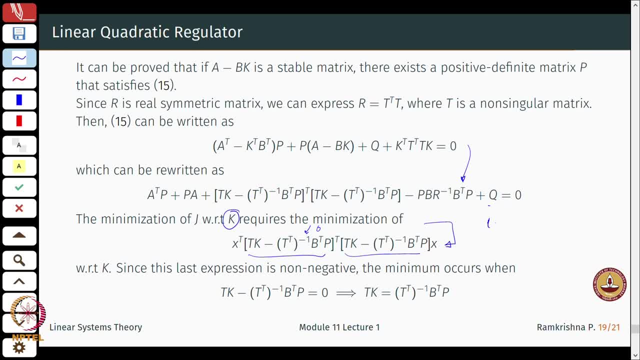 because I have something like something with the transpose and this will always be non negative. So the minimum value here is only 0, and this 0 occurs when the term in the bracket becomes 0, which essentially means that T, k is something like this: 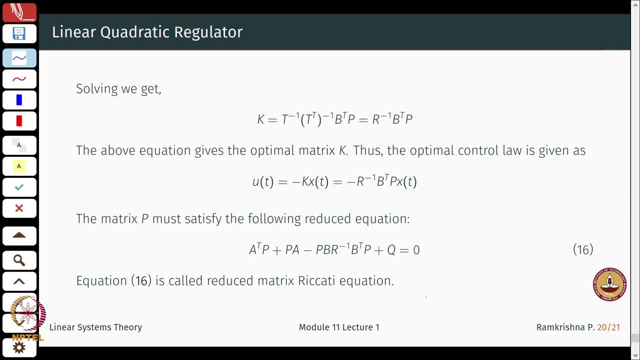 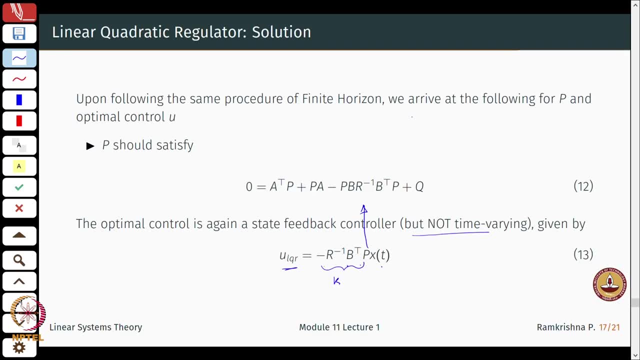 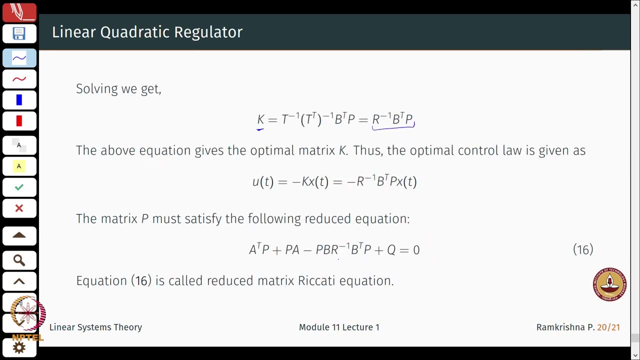 Now we can back substitute and get a good looking value of k, which is R inverse b transpose p. Let us keep this limit. R inverse b transpose p is what we also had here. this was my k here, right. R inverse p transpose p, right. So therefore.